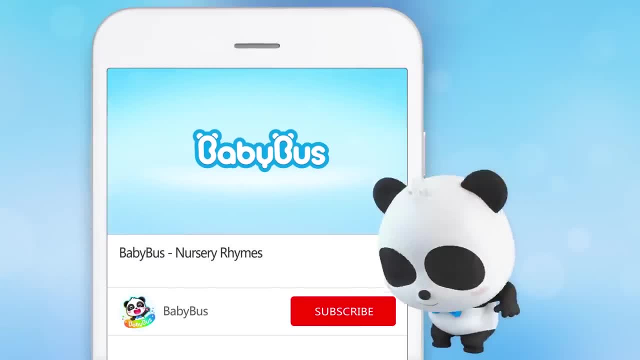 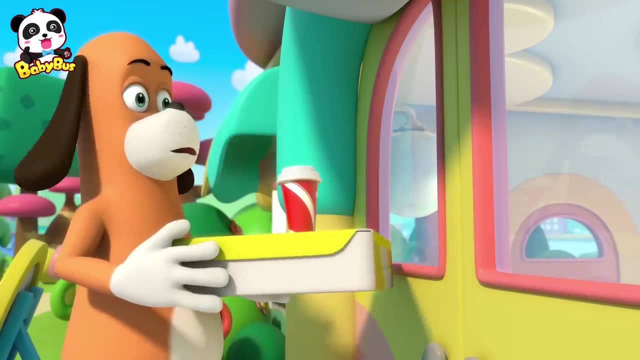 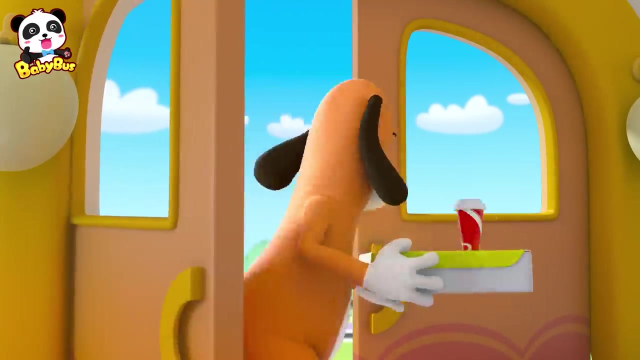 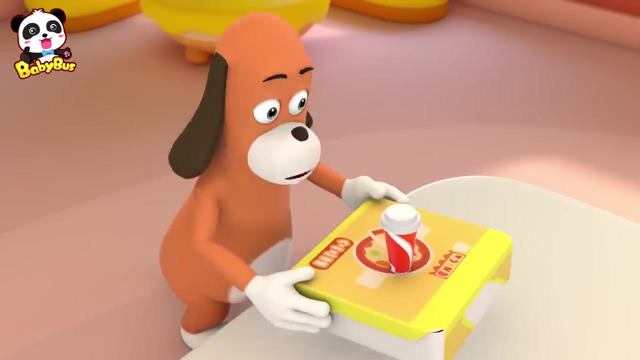 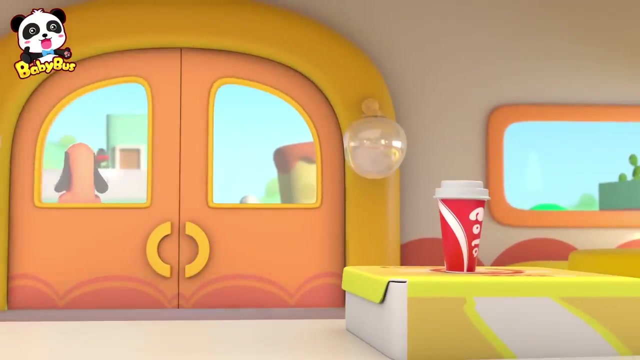 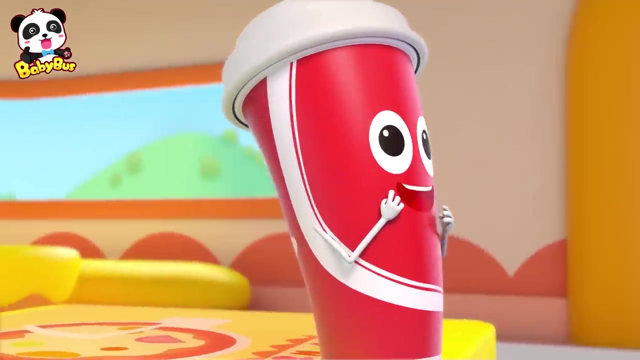 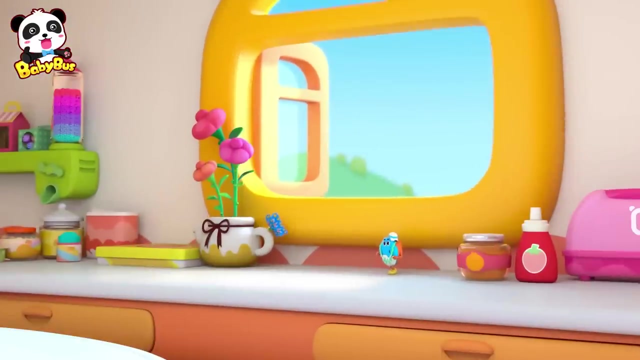 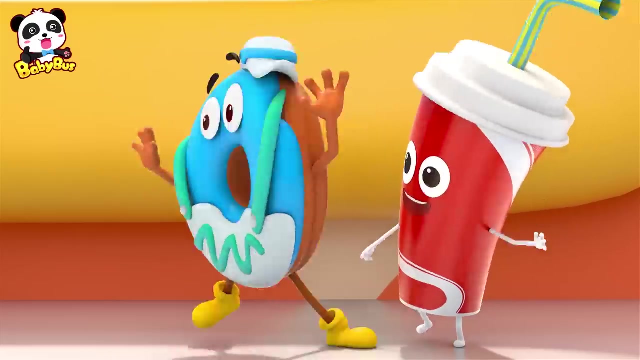 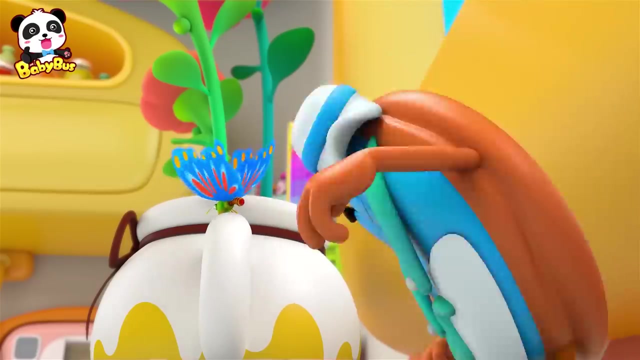 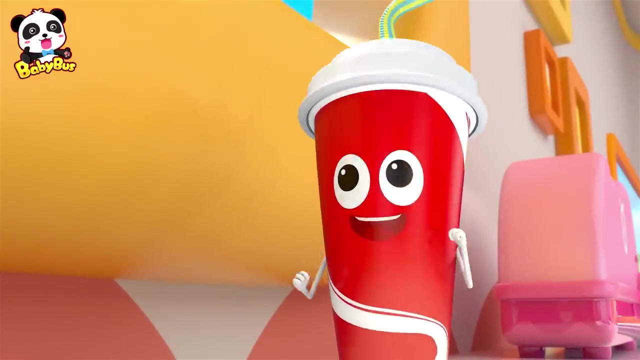 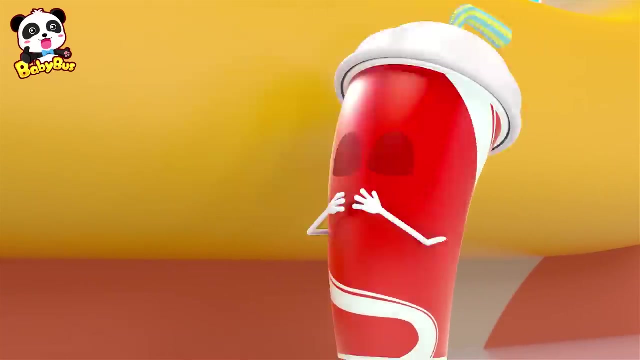 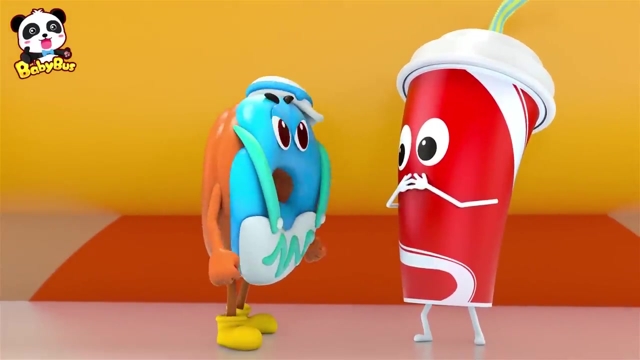 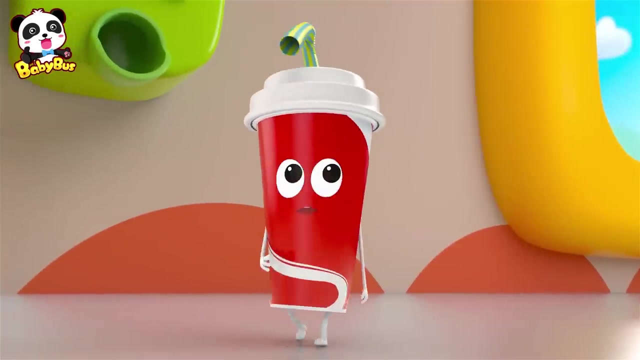 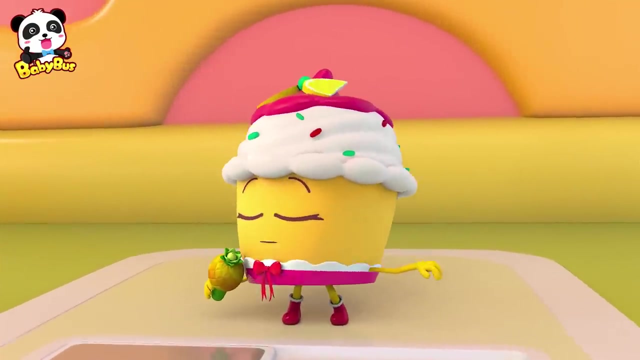 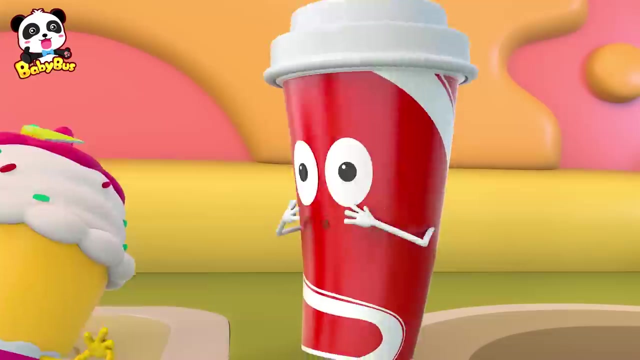 Baby bus. click here to subscribe. Your food is here, Kiki, Mew Mew, I'll just put it on the table. Oh, New friend. Oh, You scared away my butterfly, Sorry. Oh, A beautiful castle. A beautiful castle, You and me together. Such a nice voice. Hi, Let's build a castle. 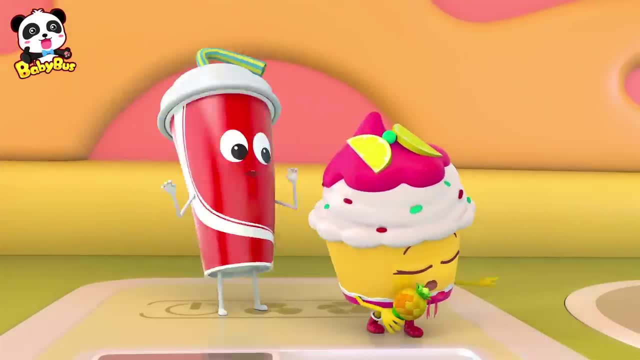 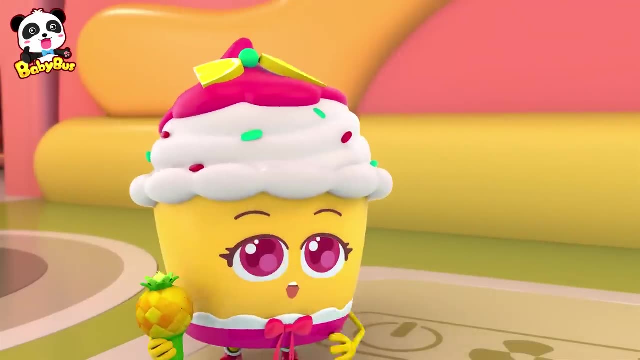 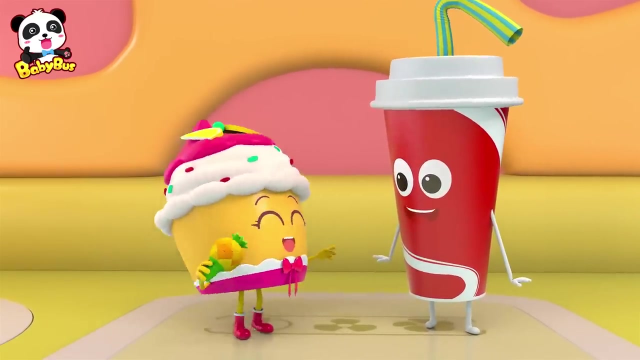 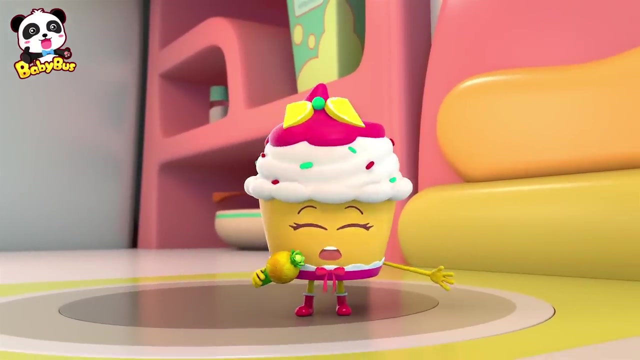 Let's be friends. A beautiful castle. Hi, I'm Kola, You and me together. Hi, Oh hi, You're a really good singer. Can you teach me how to sing? Of course, Listen carefully. La, la, la, la, la la. Let's build a castle. La, la, la, la, la la. 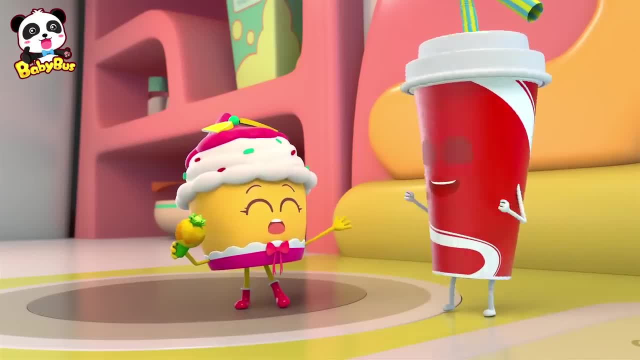 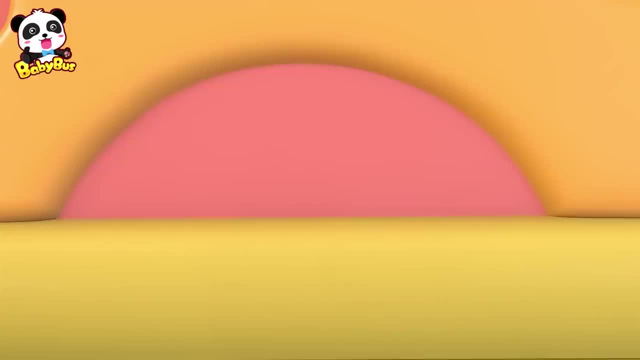 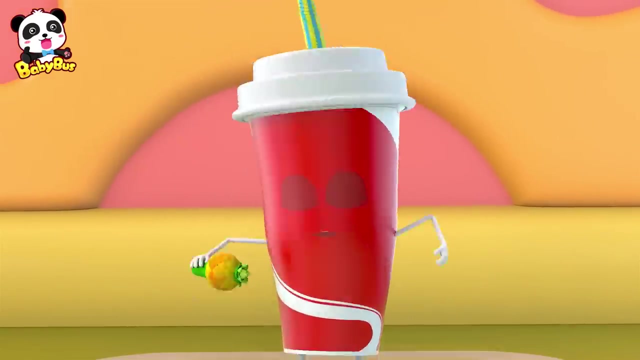 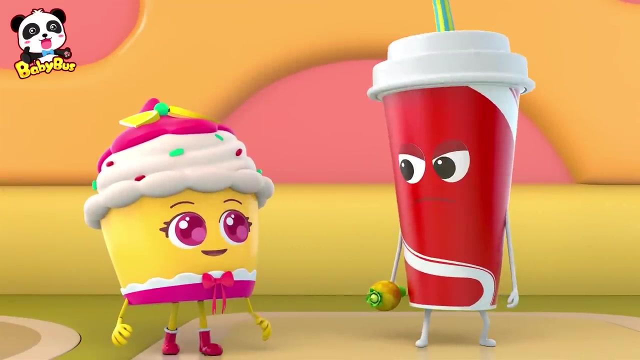 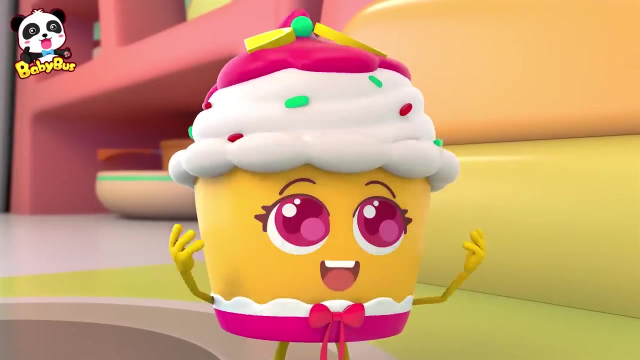 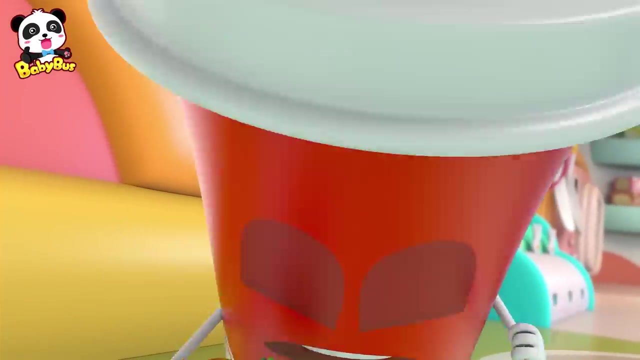 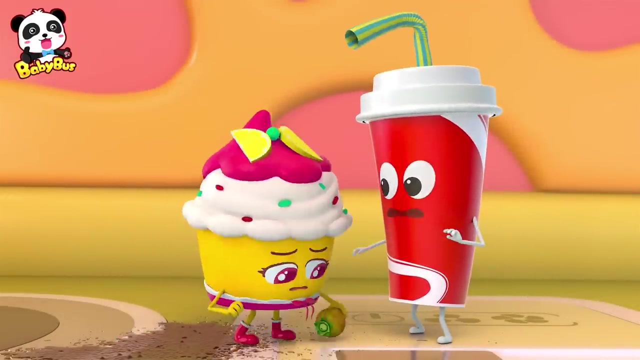 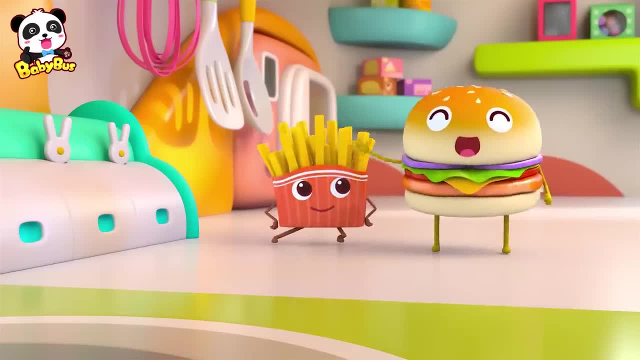 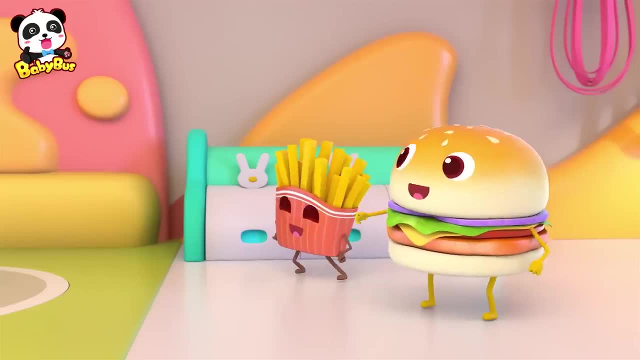 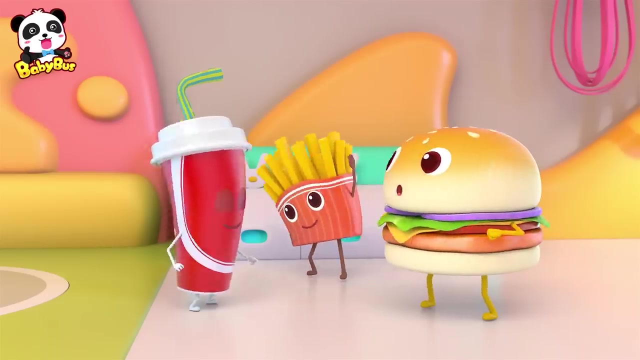 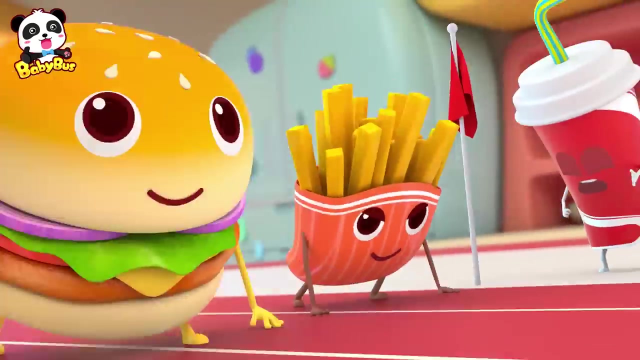 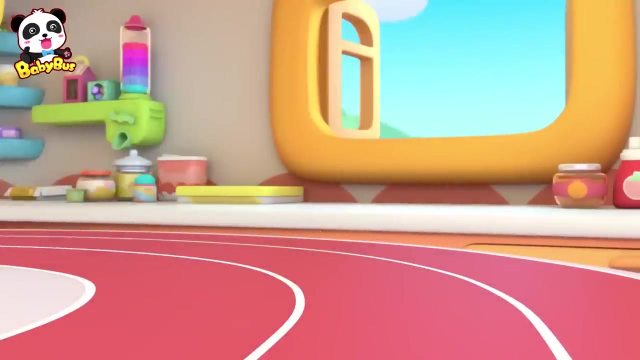 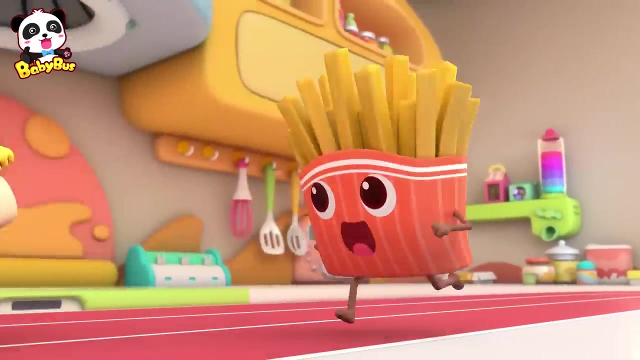 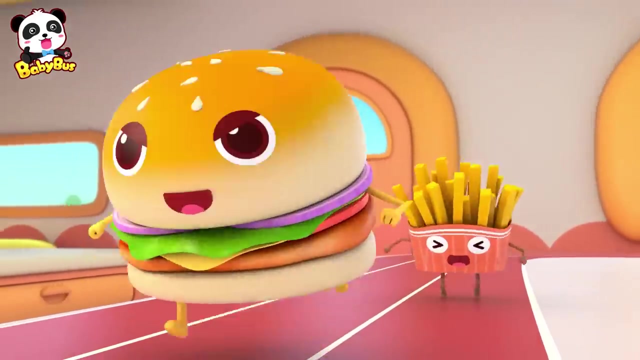 Hey new guy. Ah, Will you help us? Ah, Okay, Ah, We will have a running race. Can you be the referee? Can you be the referee? Okay, That's it. That's it, Go Run. Ah, Ah, Ah, Come on Run. Ah. Ah, Come on, Go Ah. 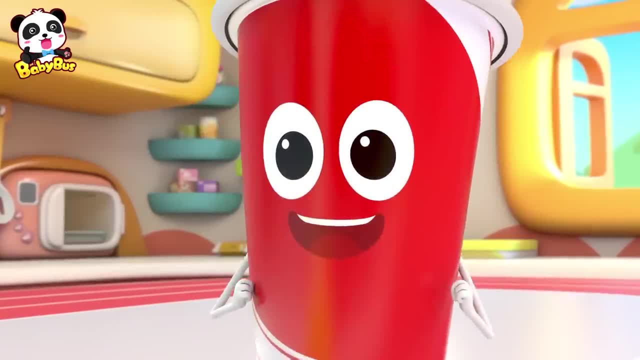 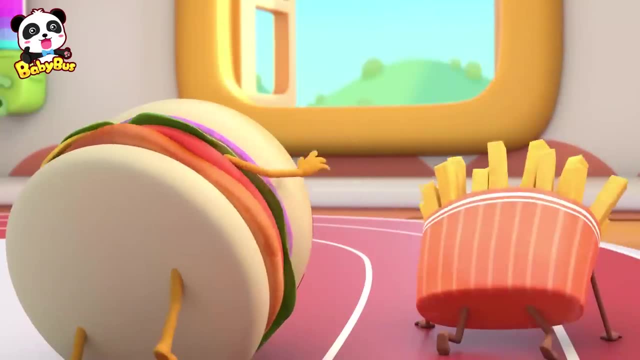 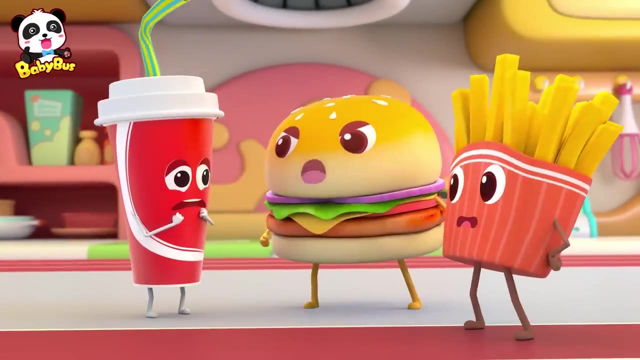 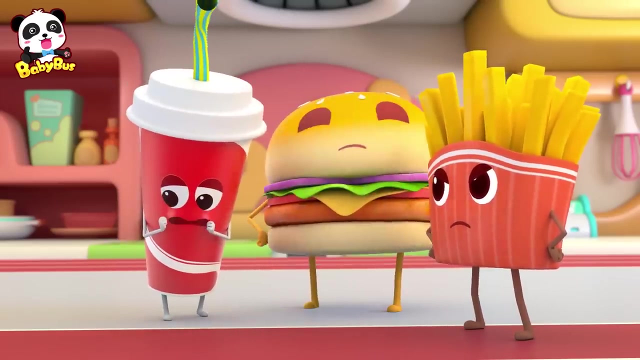 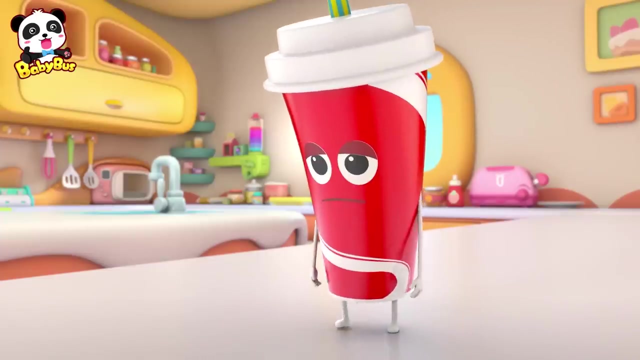 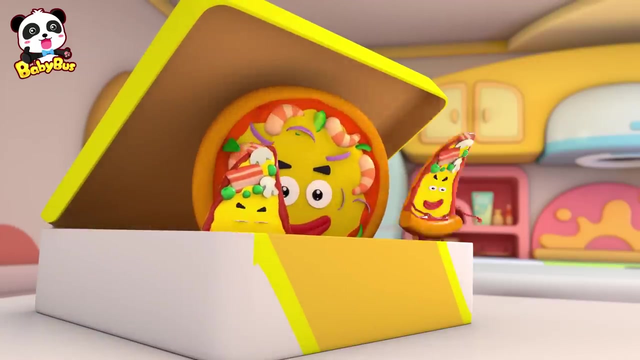 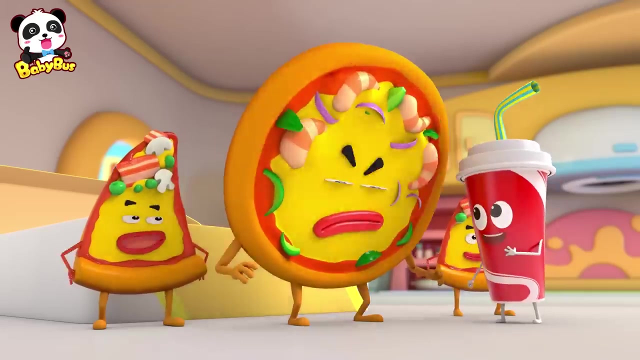 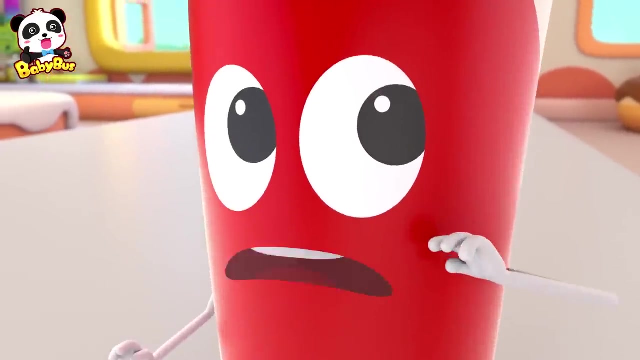 Come on Run. Ah Ah, Ah, Ouch. Hey, Sorry, I didn't mean it. You ruined our race. It's all your fault. Sorry, I burp when I get nervous. Let's go Wait. Ah, Ah, Ah, Ah, Ah, Ah. Hi, Hi guys, I'm Kola Wha. 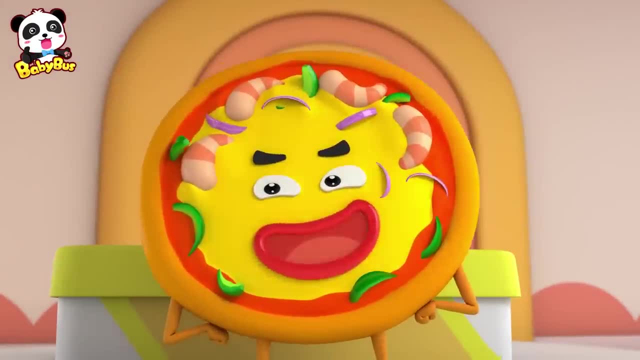 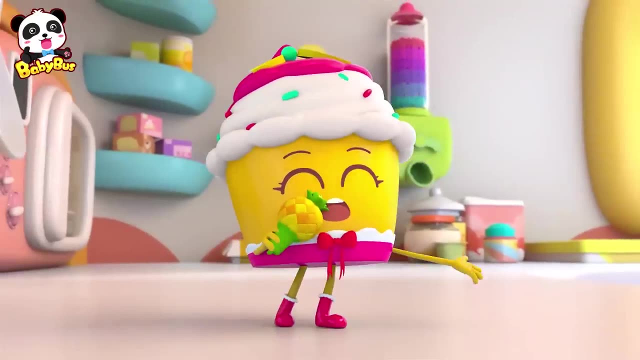 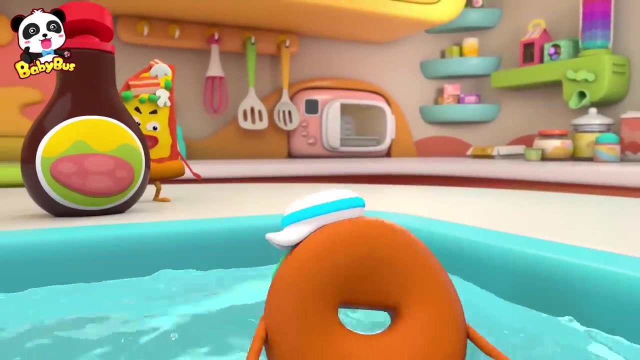 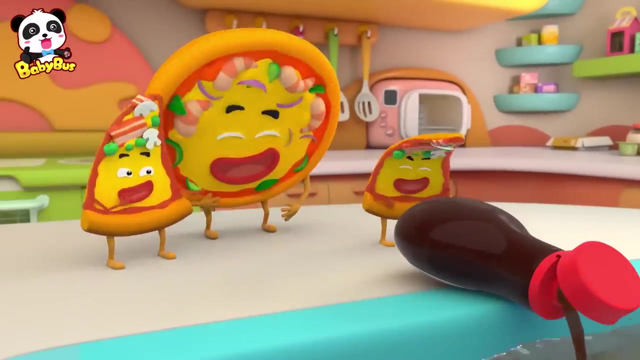 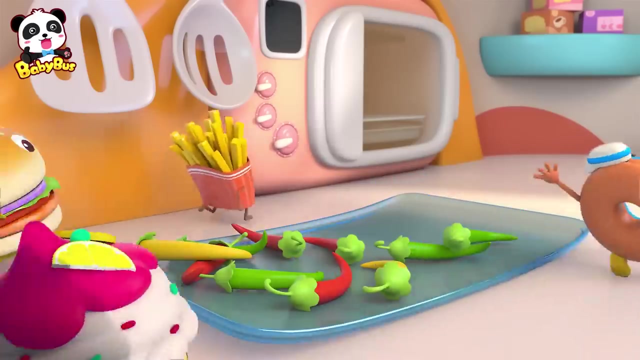 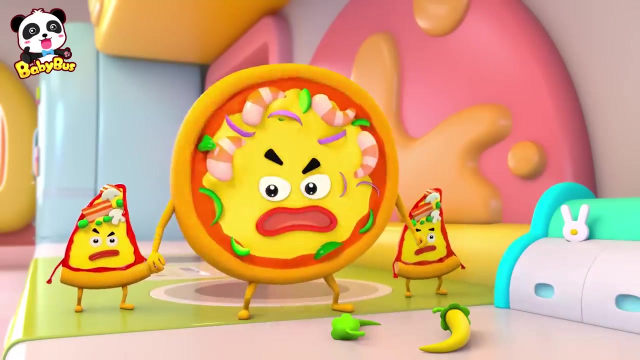 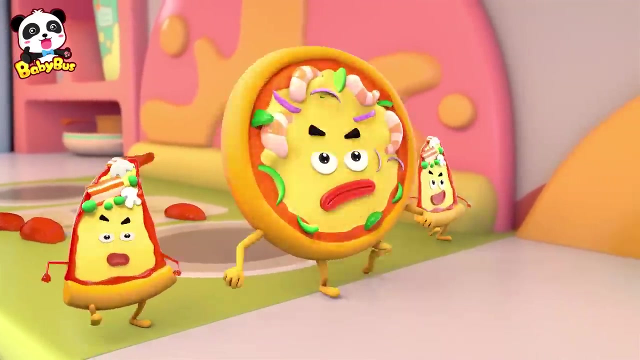 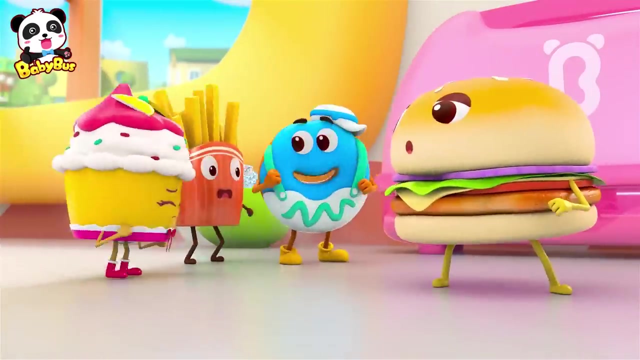 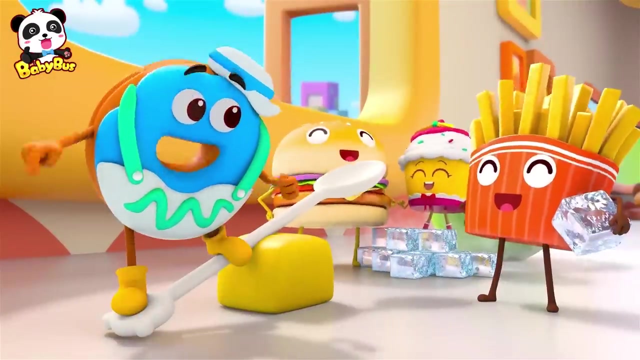 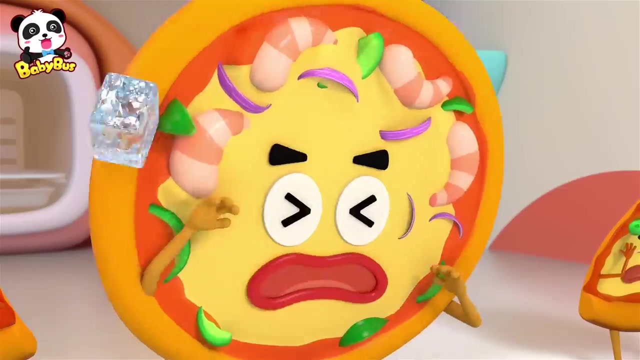 What, What are you doing? Ah, I like it here. It's all ours La, la, la, la, la, la. Ah. Ah, Take that. Oh, I have an idea: Ice Cube Bob. Oh, Oh, Oh, Oh, Oh, Oh, Oh. 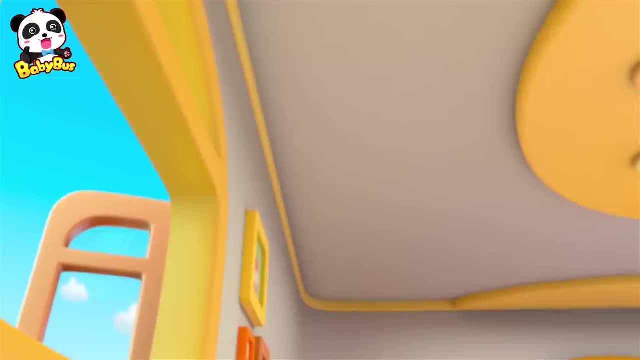 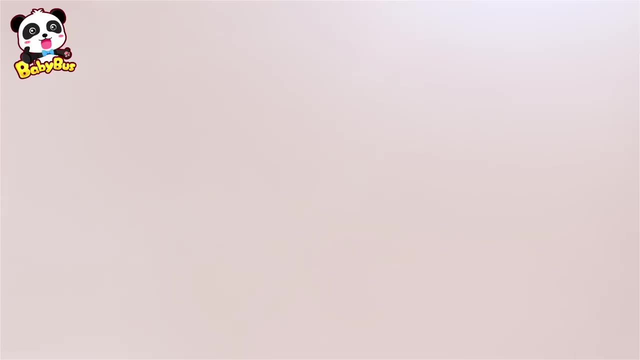 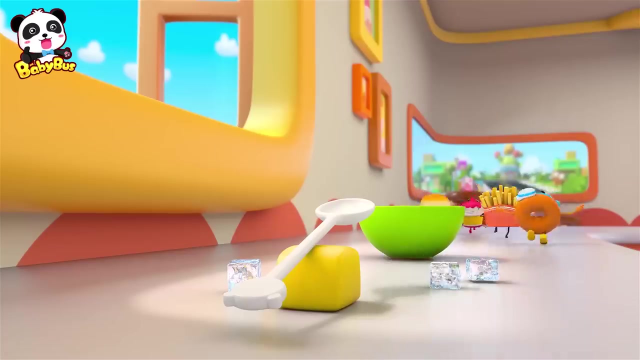 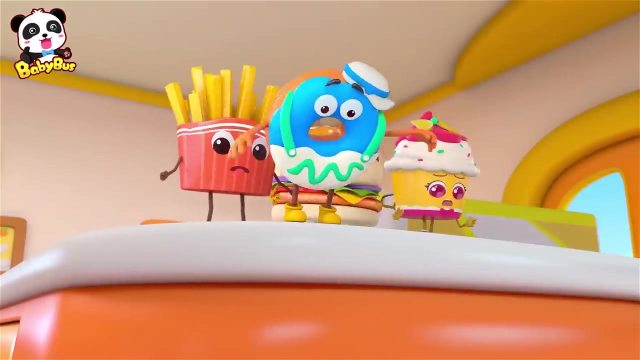 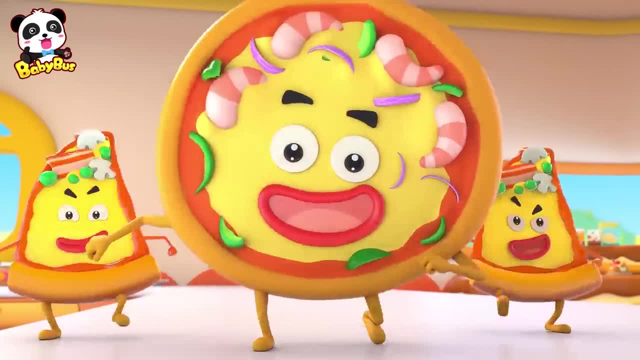 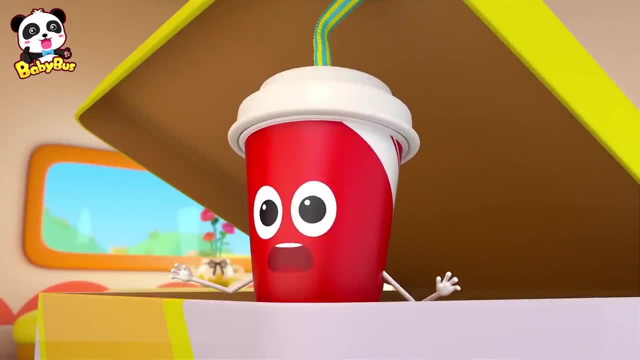 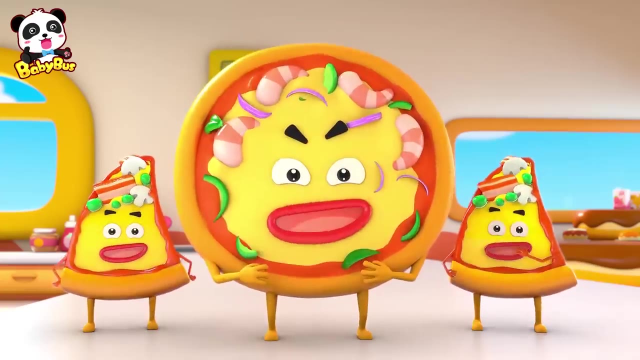 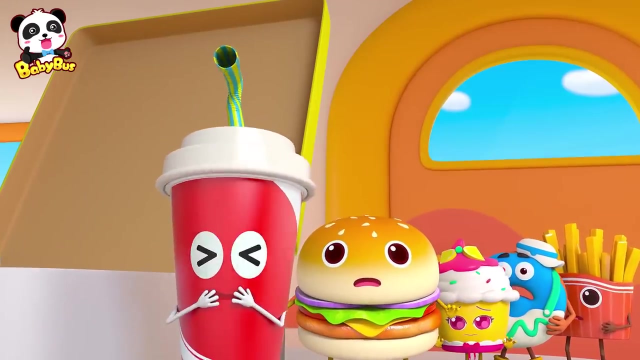 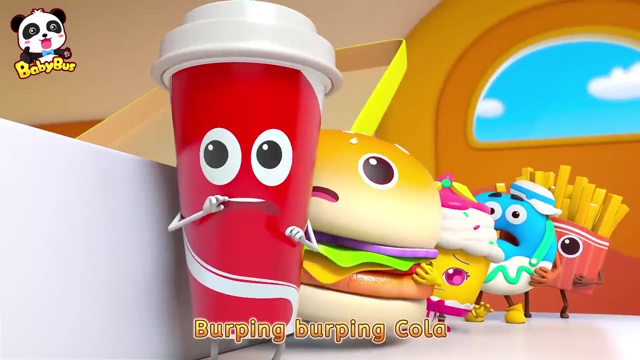 Relax college bodyguards. That's what I'm saying. Ha Ha, Ha, Ha Ha. Stop You again. Stop, Don't come any closer. Burping, burping cola, Burping, burping cola. 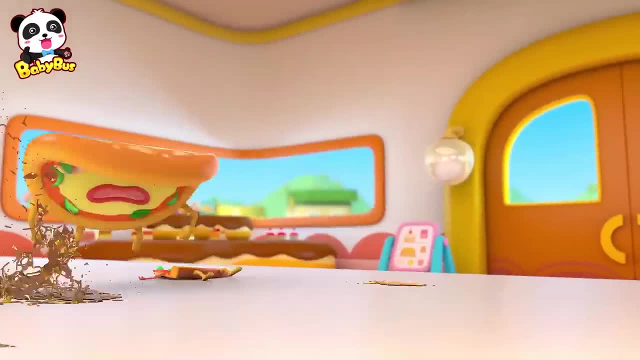 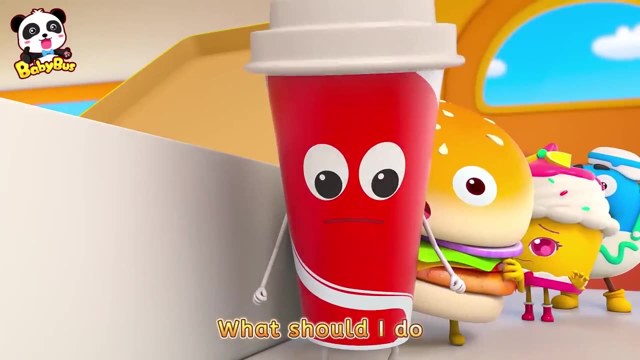 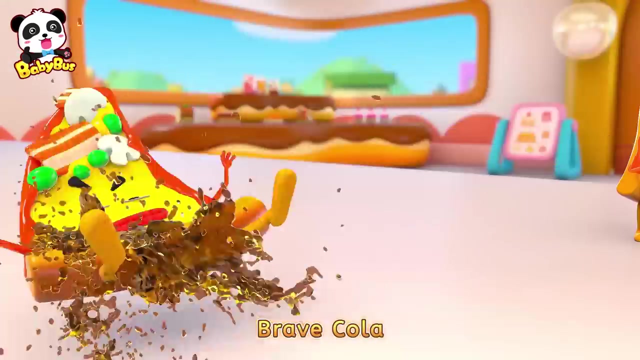 Burping, burping cola. Three bad pizzas make a mess. Brave Cola says: what should I do? Let's see what we found out. Cola bomb, Come on, come on, Brave Cola. Cola bomb, Boom Cola bomb. 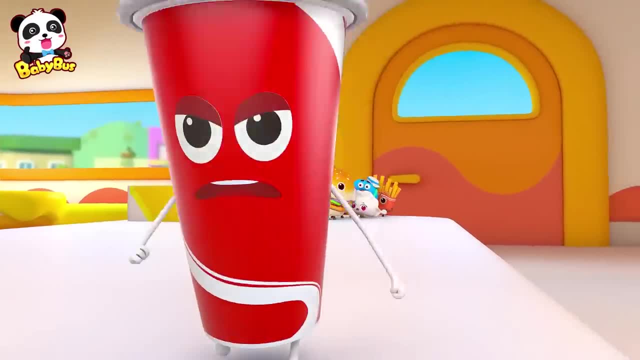 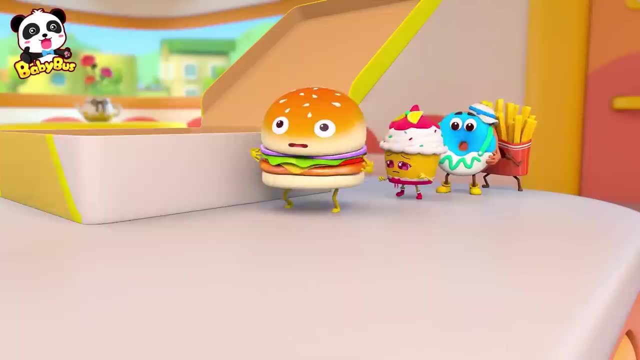 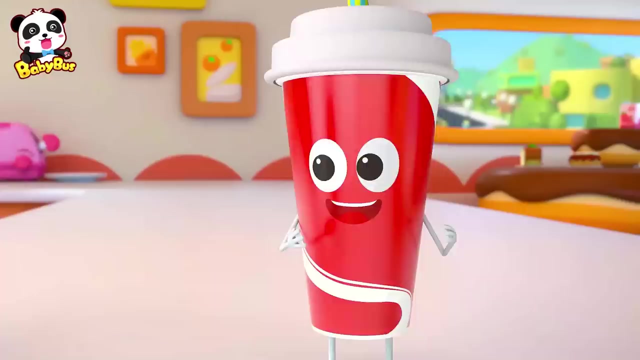 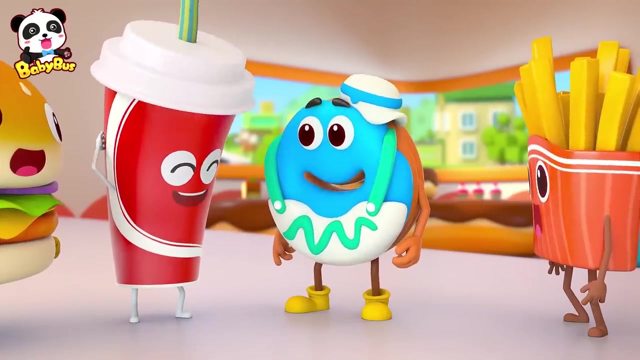 Boom, Here we go. here we go. Brave Cola Burping, burping cola, Burping burping cola, Burping, burping cola. He had the idea. Great, Thank you for saving us. Your cola bomb is so cool. 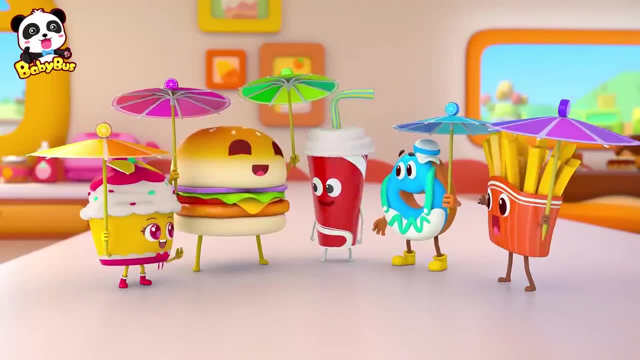 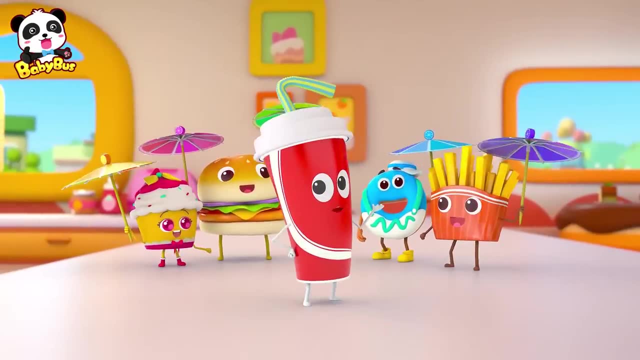 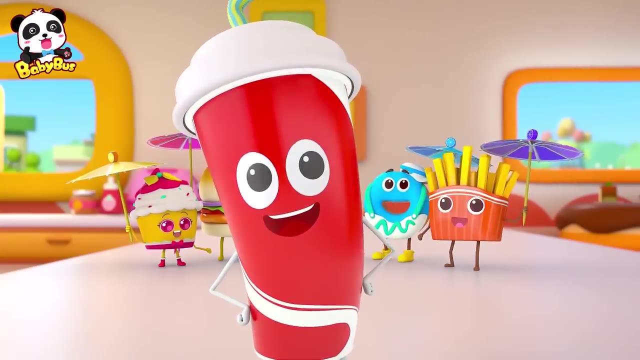 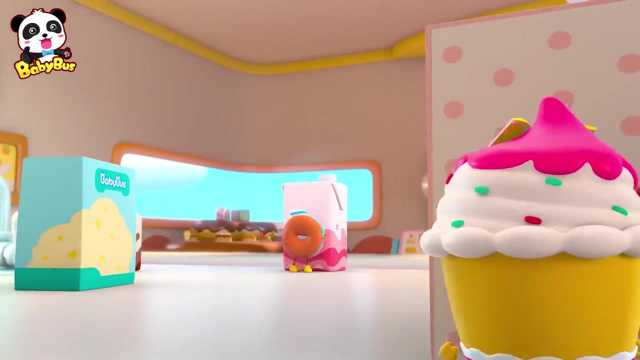 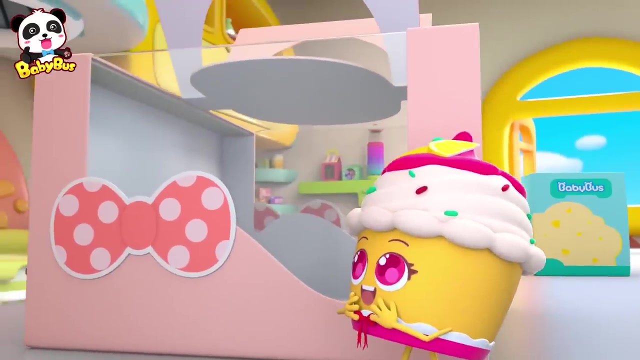 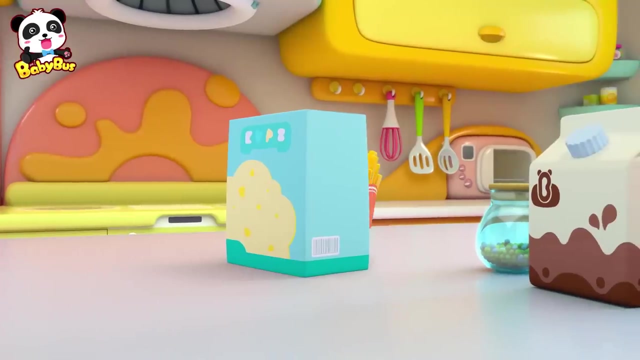 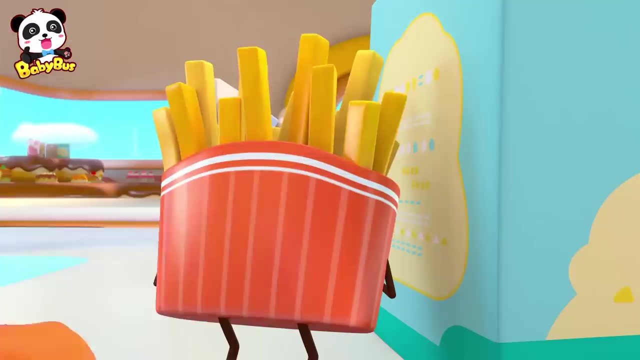 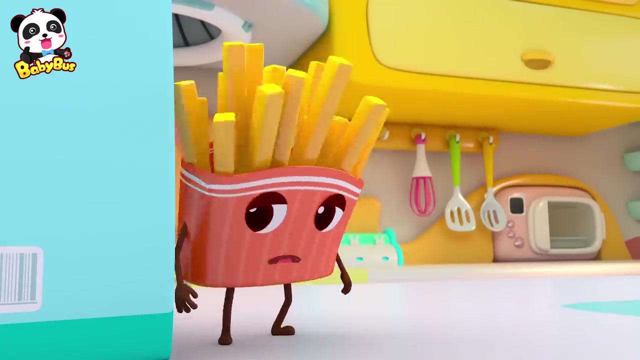 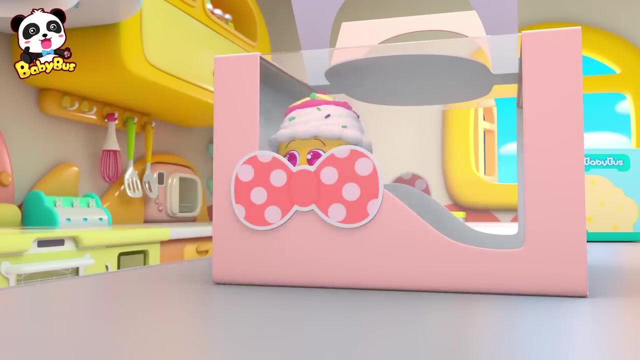 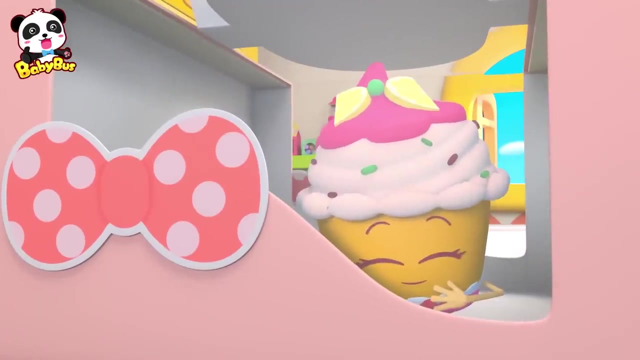 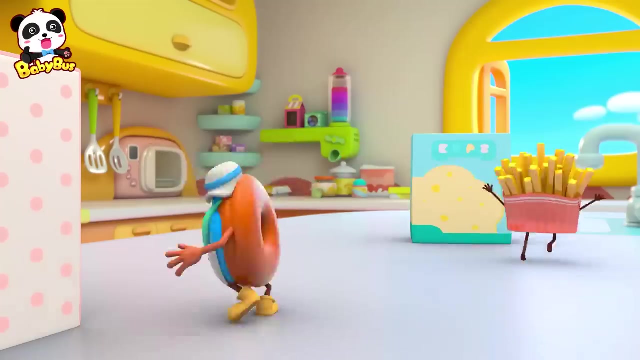 when i burp, i can help others too. kids, do you want to be friends with me? one, two, three, four, five, huh, are you ready? ready or not? here i come. i found you. you got me so quickly. oh, where is katie? i can't find her. 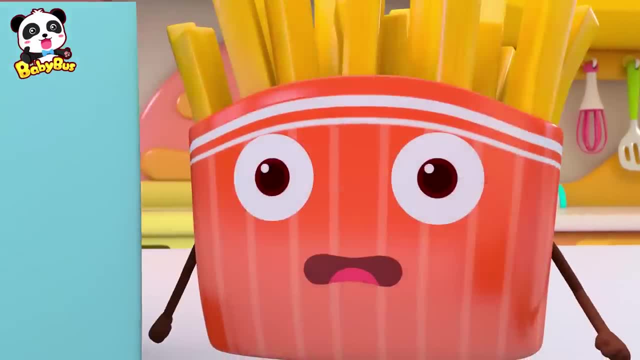 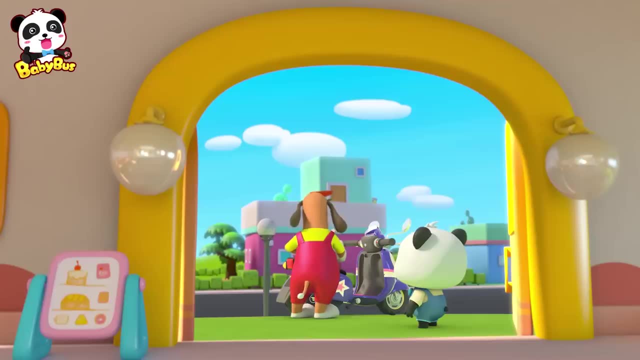 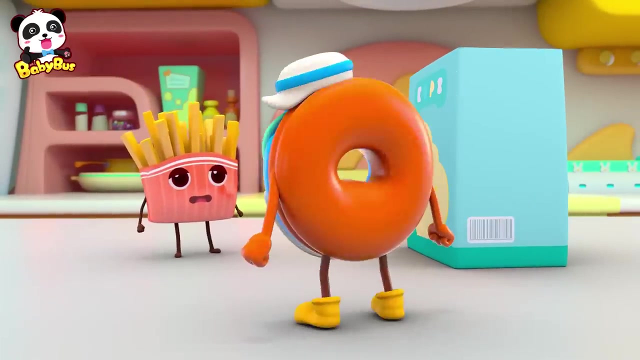 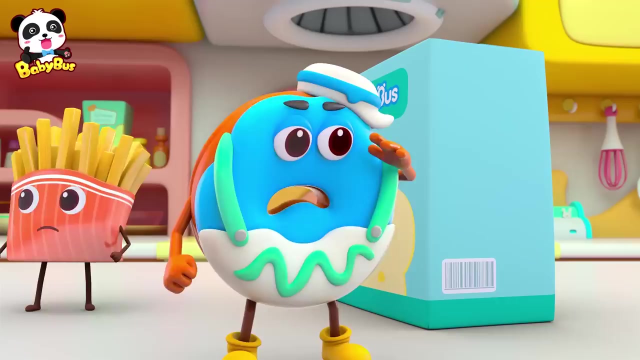 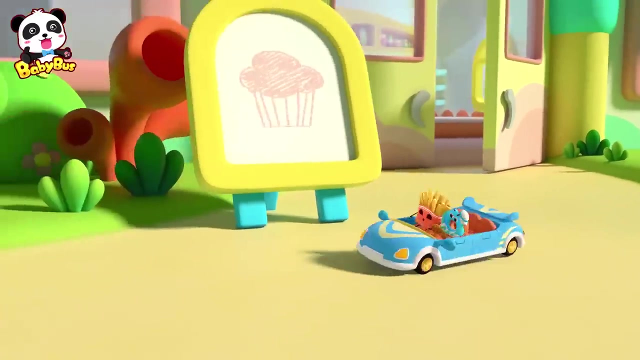 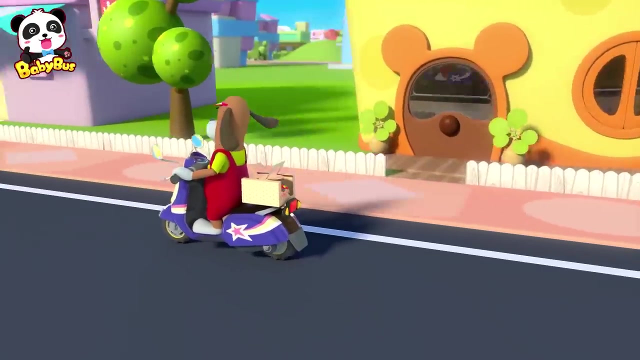 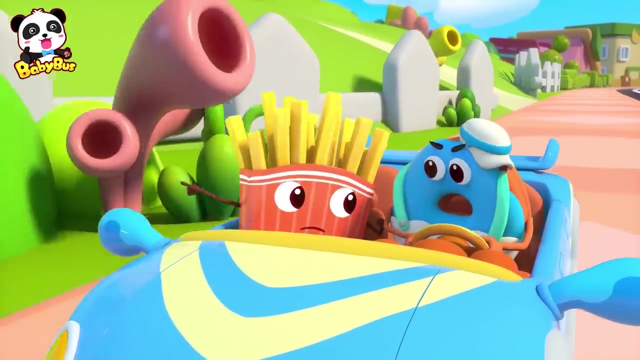 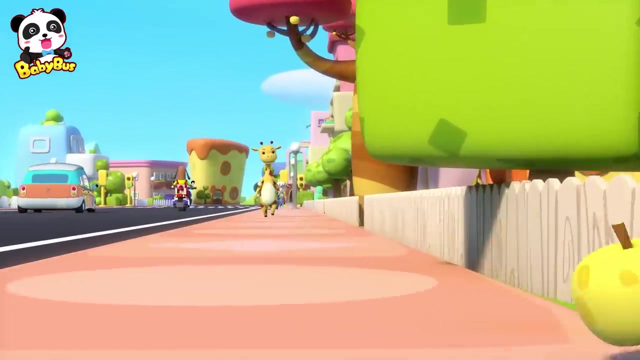 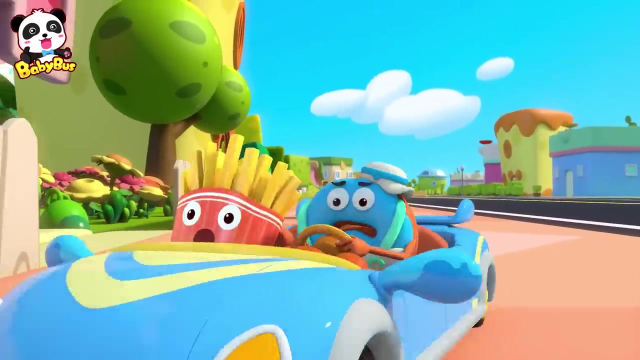 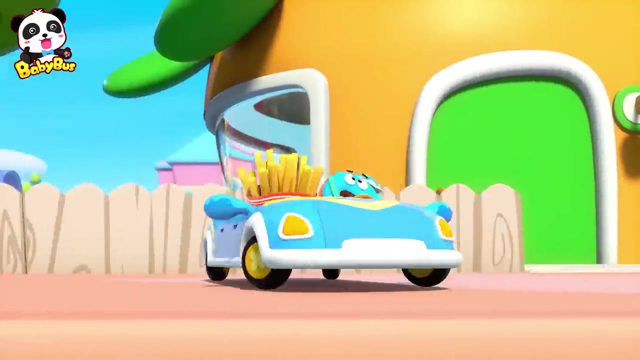 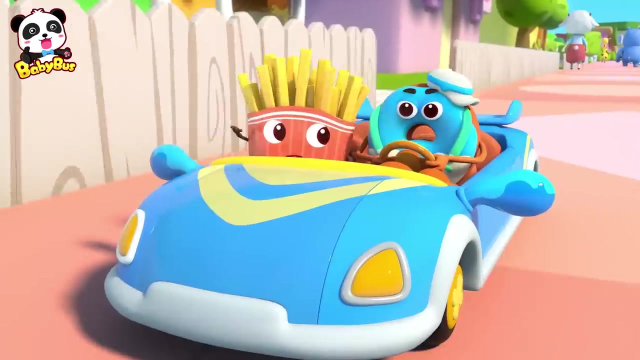 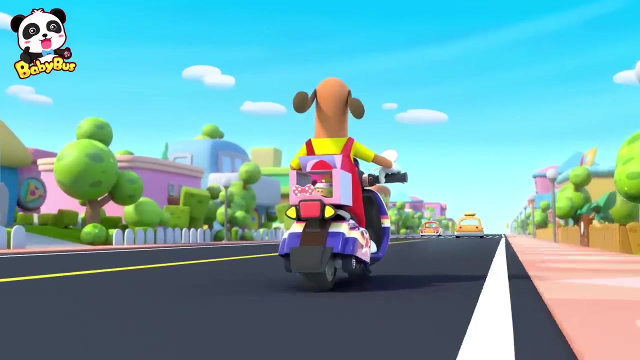 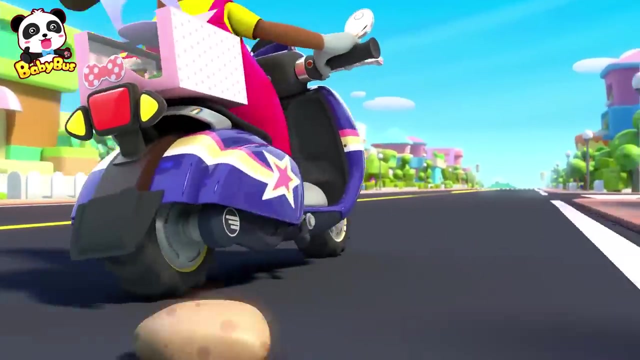 hmm, please deliver this cake to rudolph, okay, no problem. oh no, katie is in the box. what should we do? that's it. let's go save her. ah, over there, hurry up, no problem, full speed ahead. ah, come on, turn right, go, go go. oh, oh ouch. 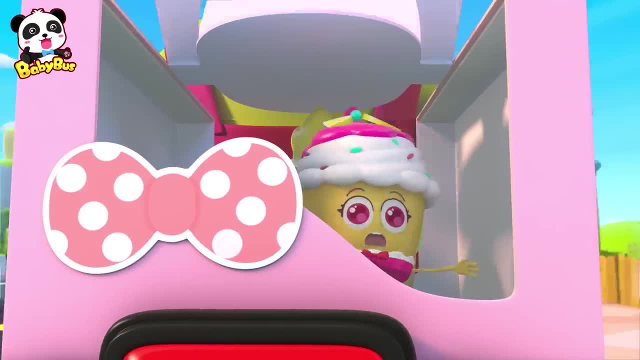 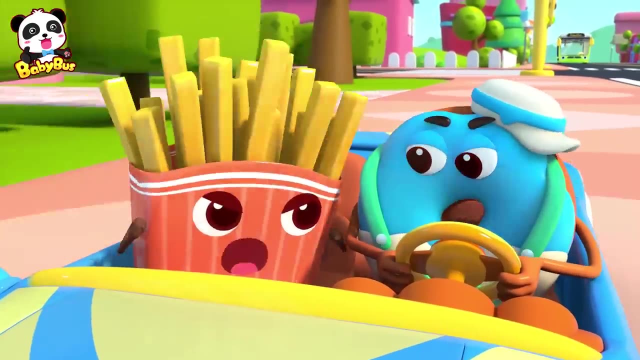 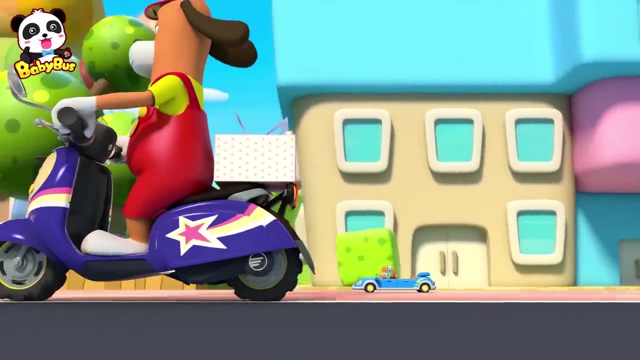 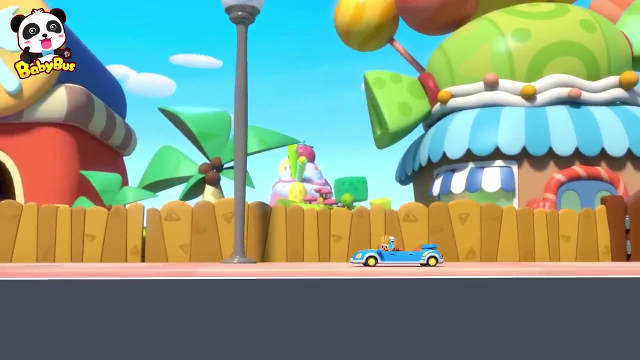 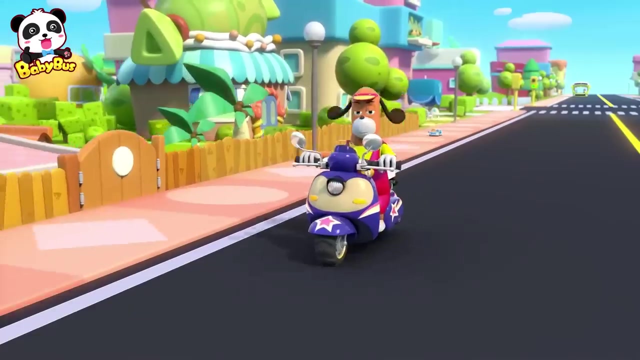 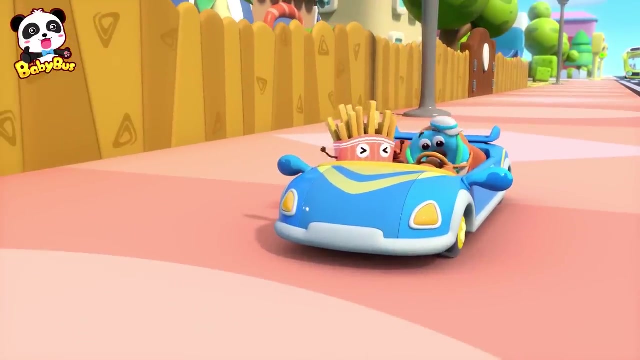 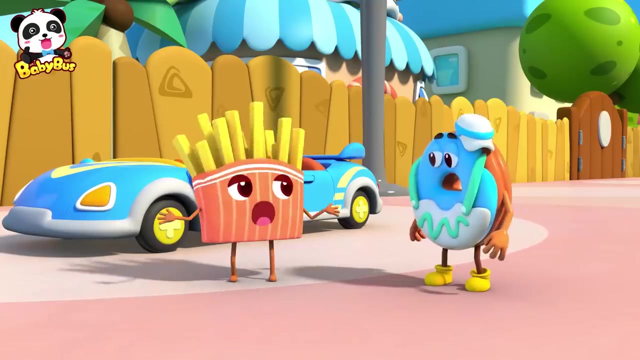 Donnie Rye Here, Save me. Yay, We're almost there Faster. Trust me, I'm really good at driving. Hurry, We need to speed up. Oh no, We're out of battery. What should we do? We won't be able to get Katie. 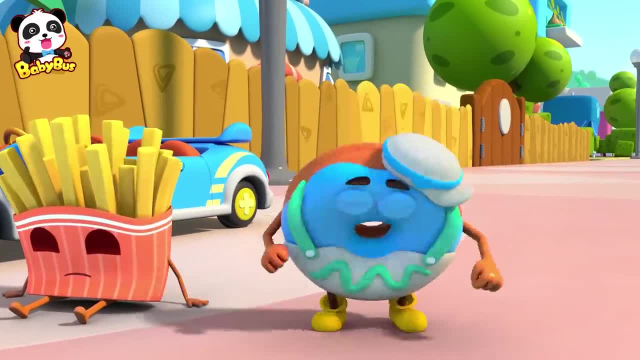 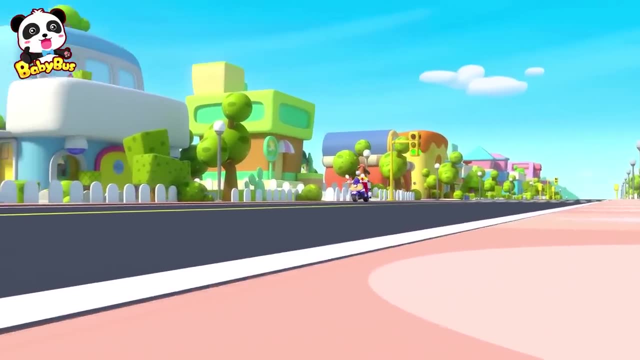 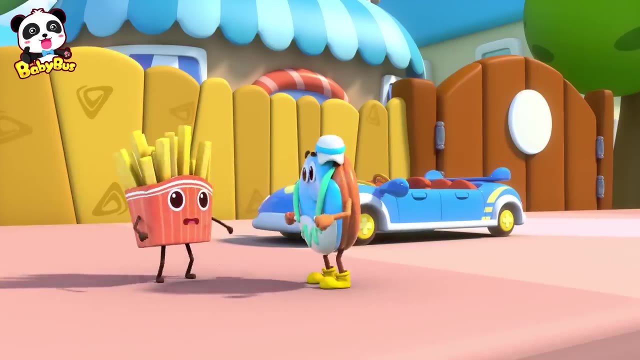 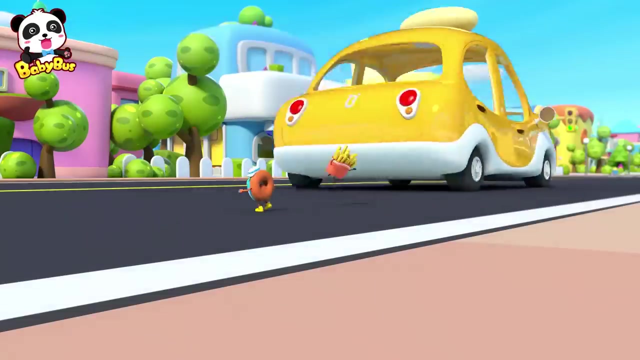 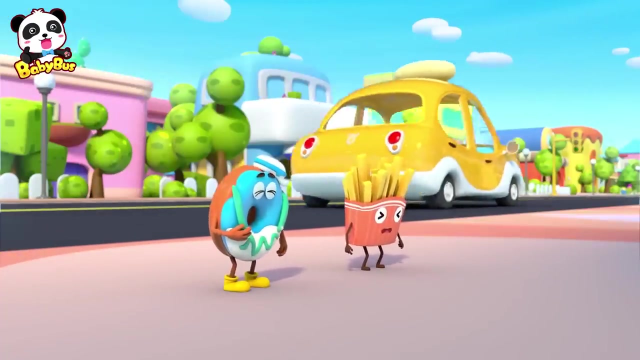 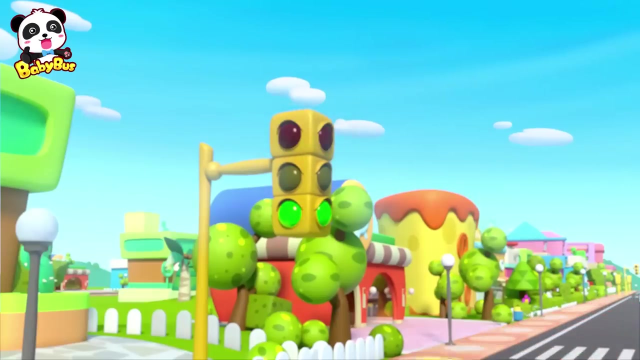 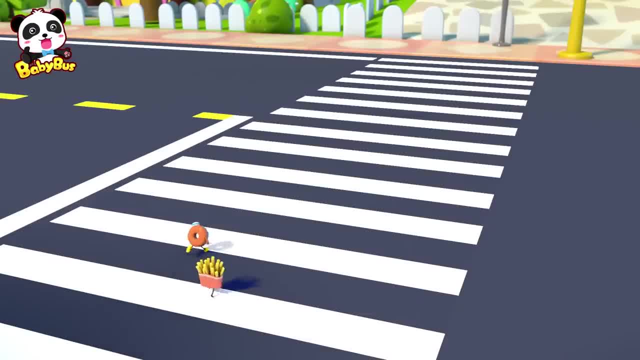 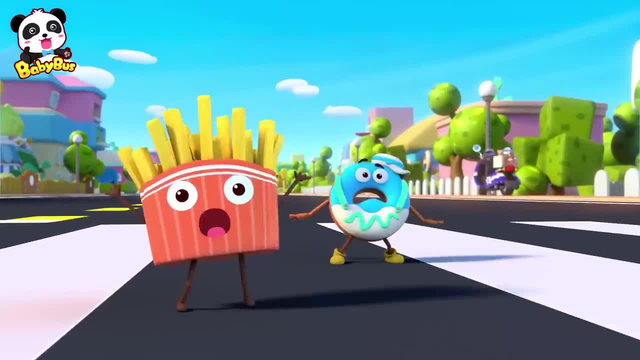 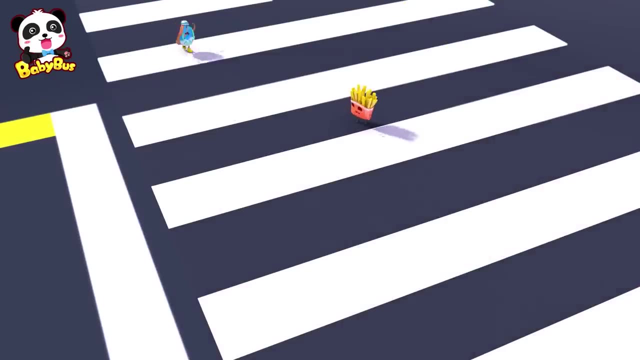 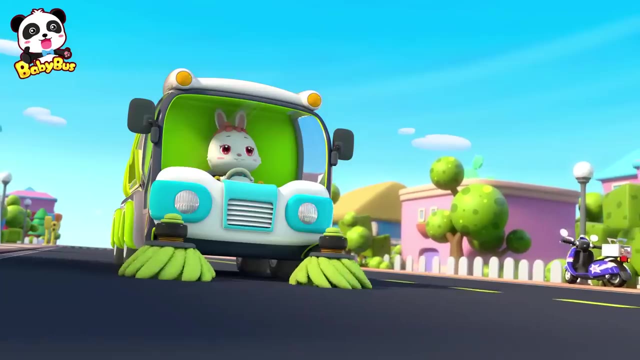 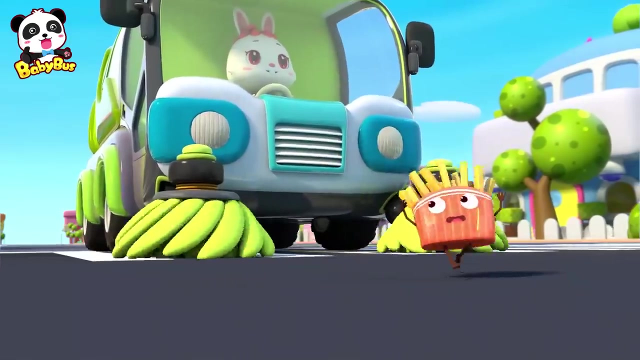 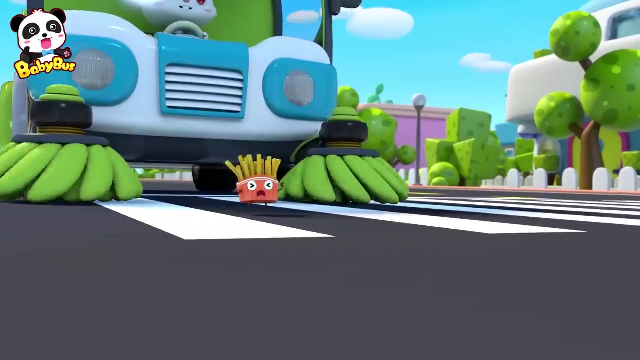 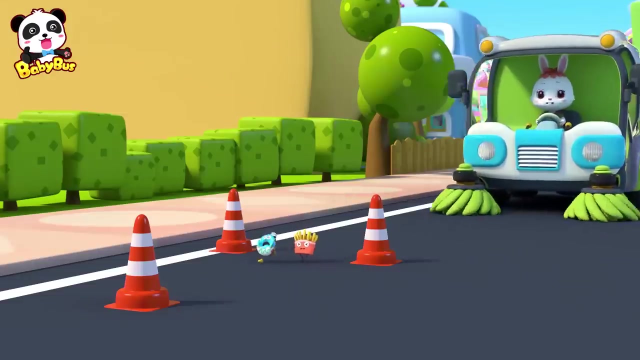 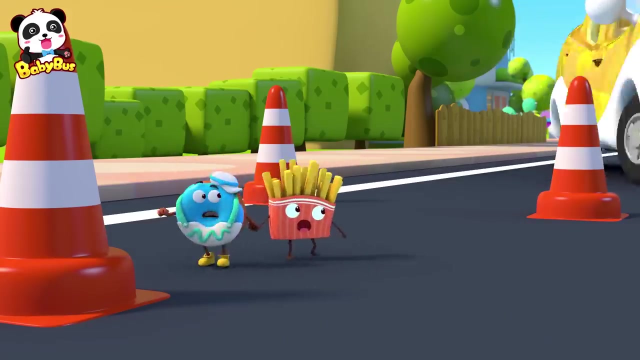 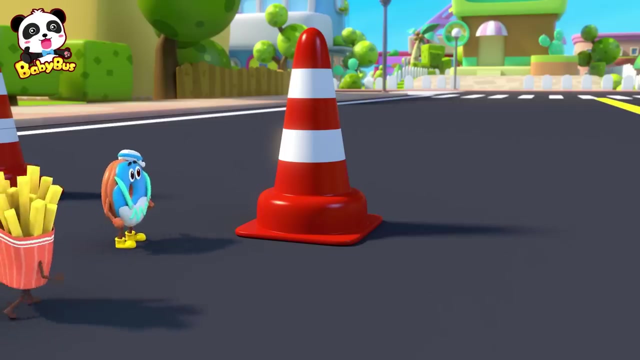 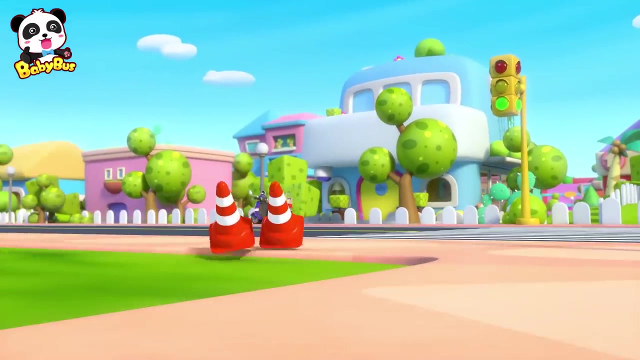 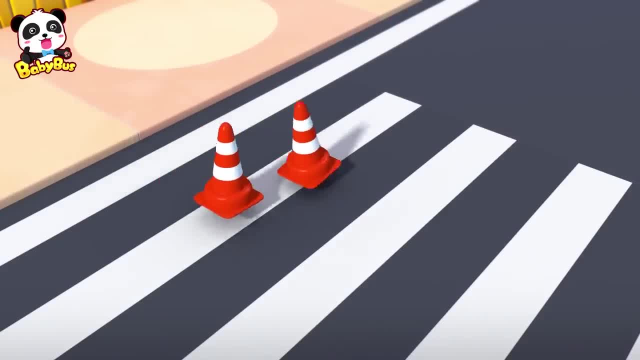 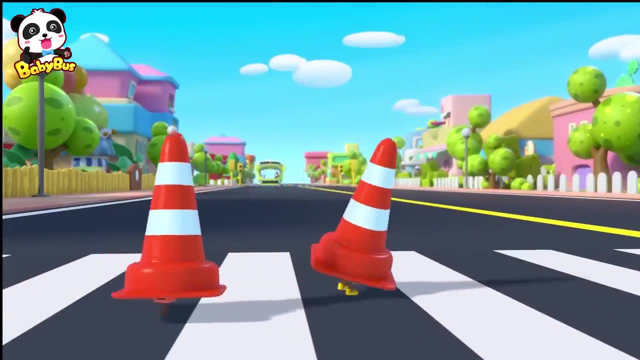 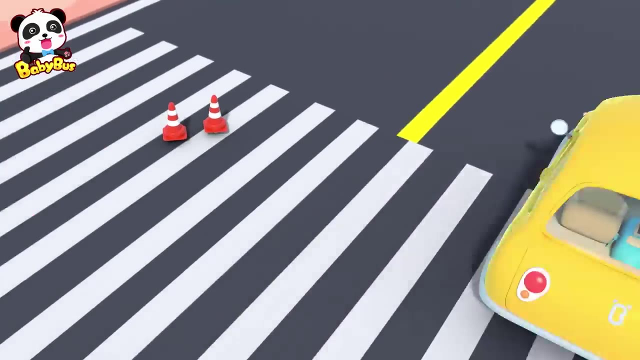 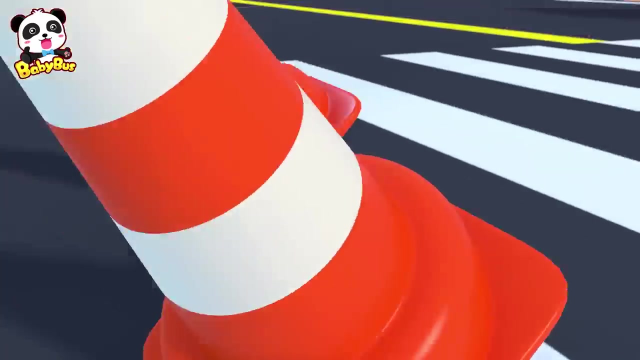 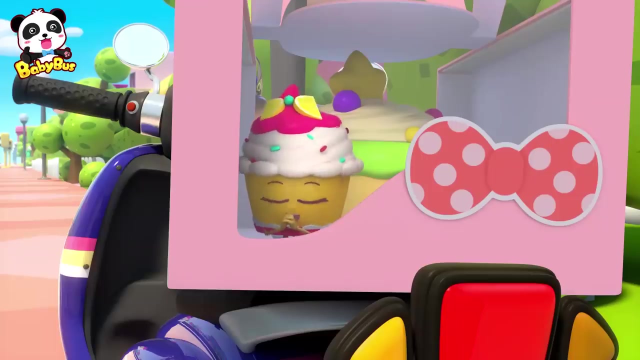 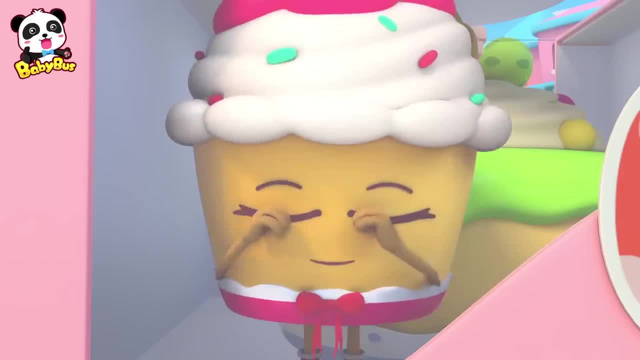 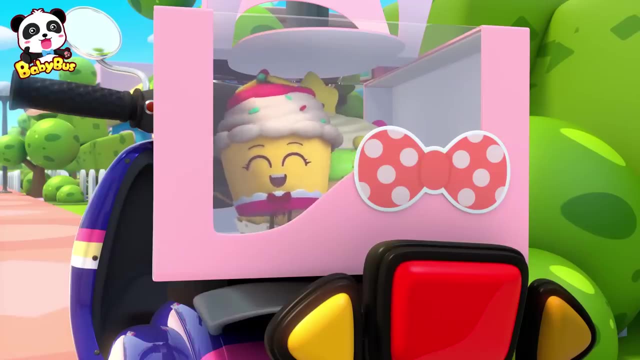 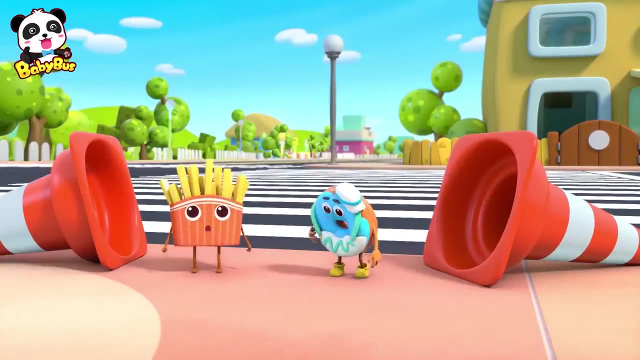 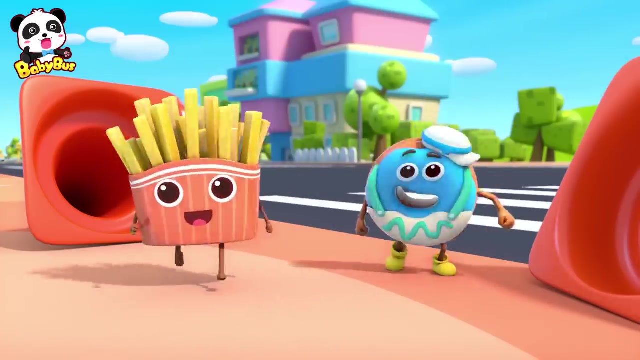 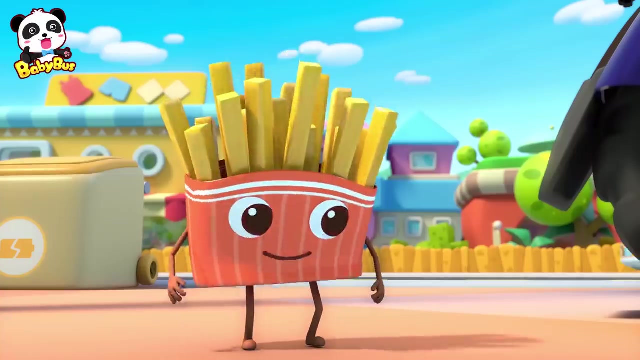 Huh, Donnie Fry. Hey, I'm here. That was so scary. It's Katie. We're here to save you. Thank you, guys. I knew you would come and save me. Of course, We're good friends. 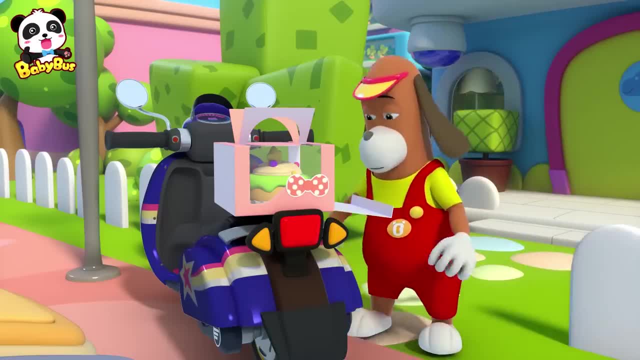 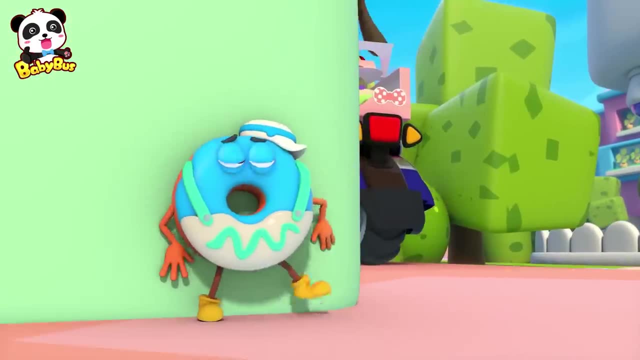 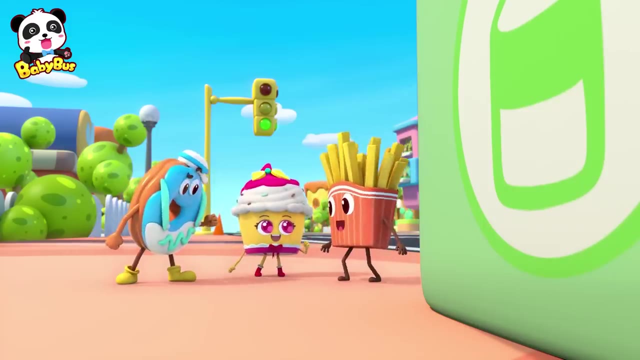 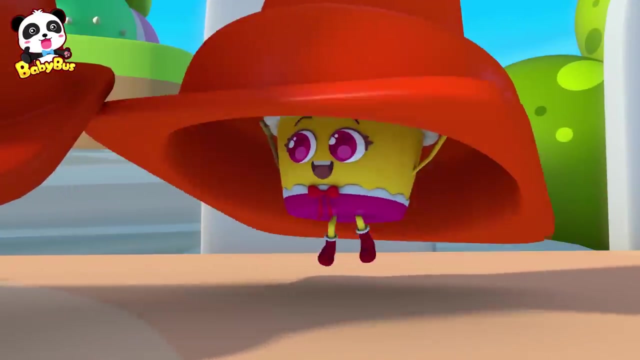 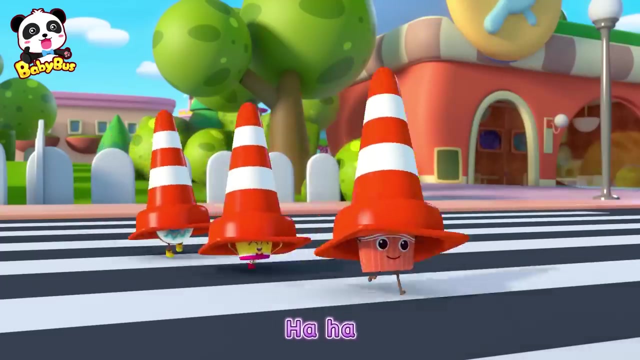 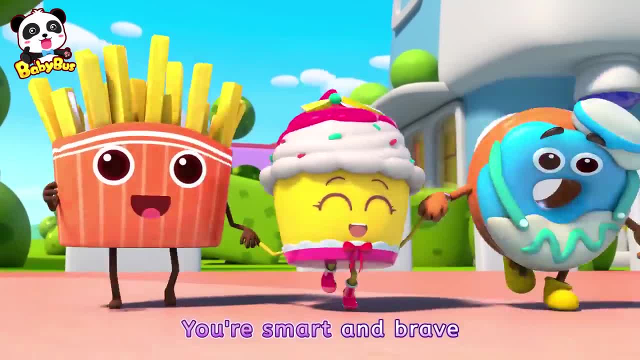 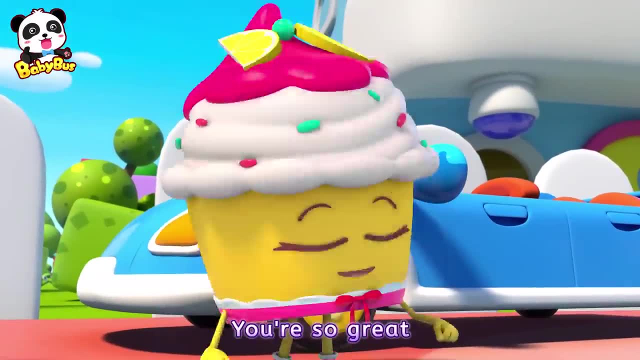 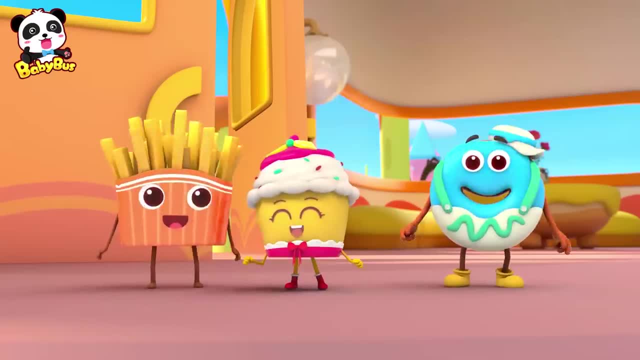 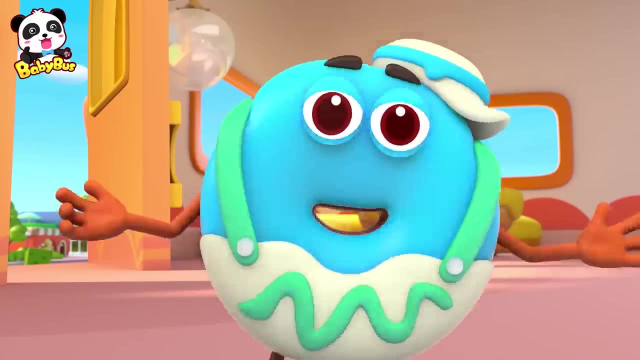 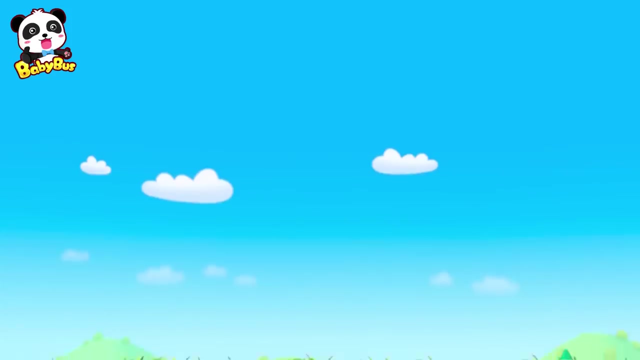 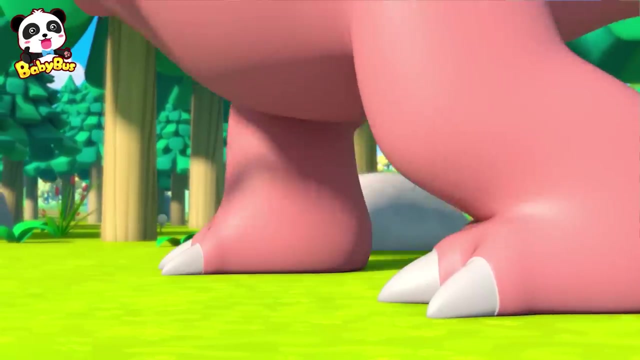 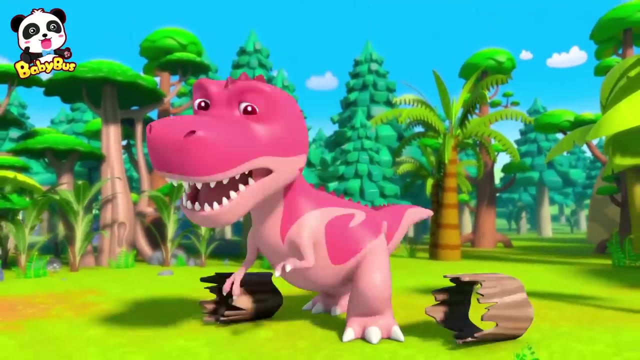 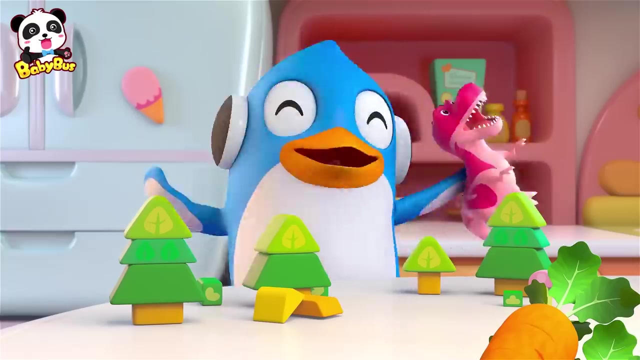 Huh, Yay. If your friends are in danger, be brave and think of a way to help them, But always remember to be careful. Arrgh, Arrgh, I'm a scary T-Rex. T-Rex is coming. 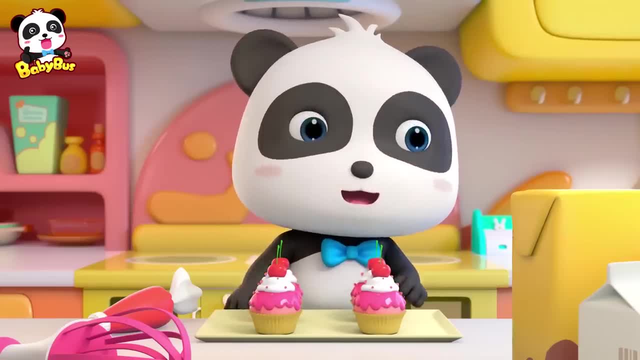 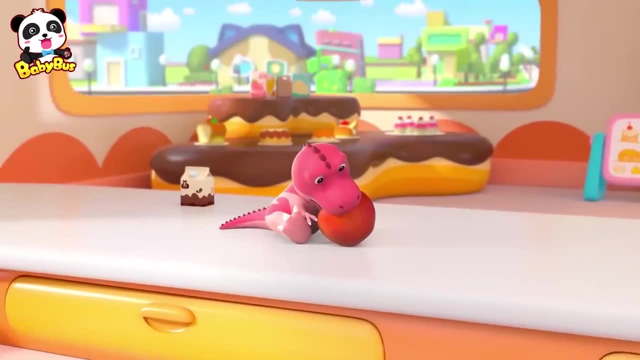 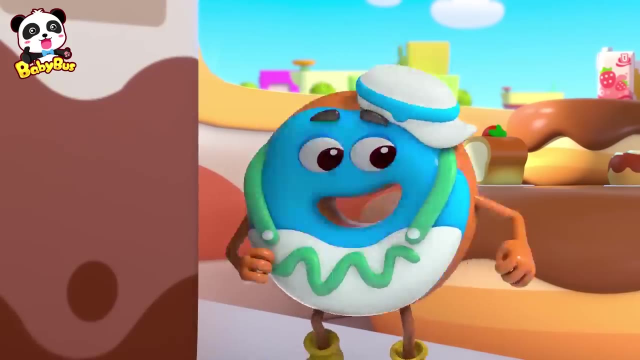 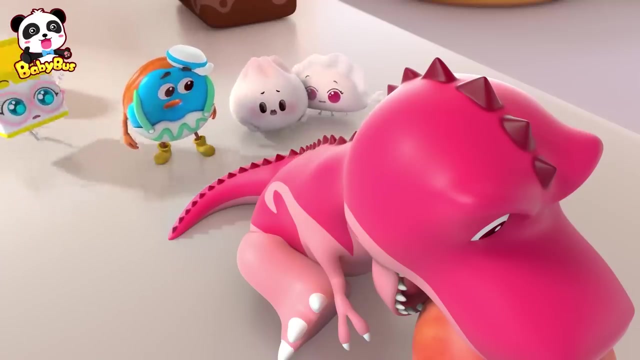 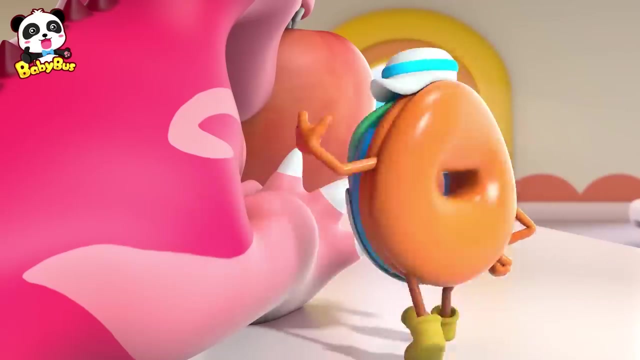 All done, Rudolph, let's go to the party. Okay, let's go. Come out everyone. Wow, It looks so scary. Look at its big mouth. It will eat everything inside. Don't be so scared, It's just a toy. 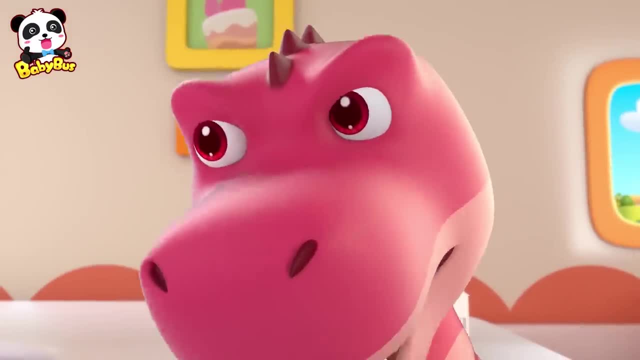 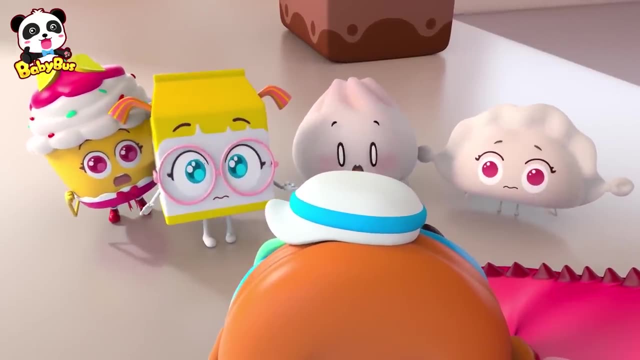 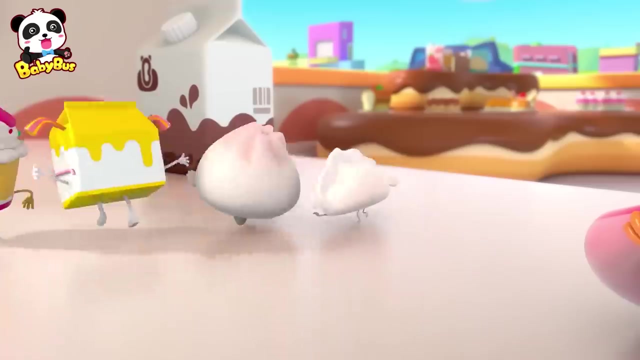 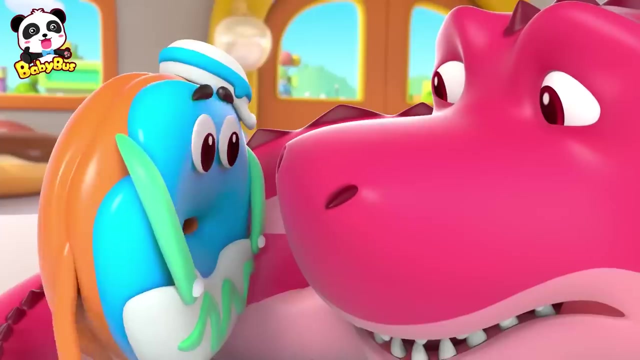 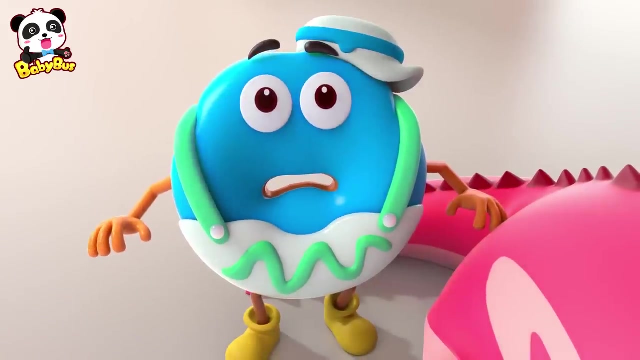 Don't be afraid, Come on, T-T-T-Tonny, It's okay, Come and touch it. No, No, Why are they running away? I'm so sorry. I just Arrgh, Arrgh, It's alive. 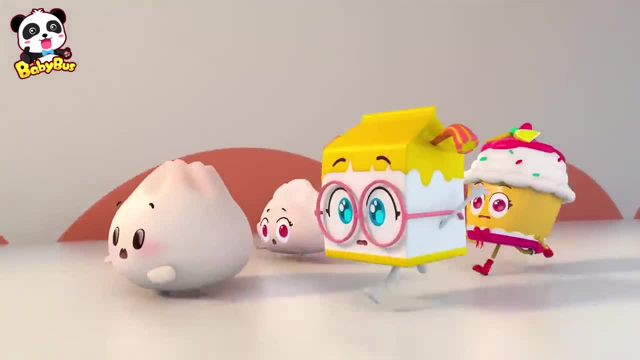 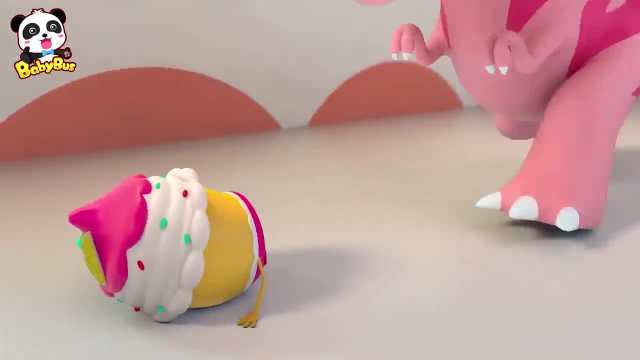 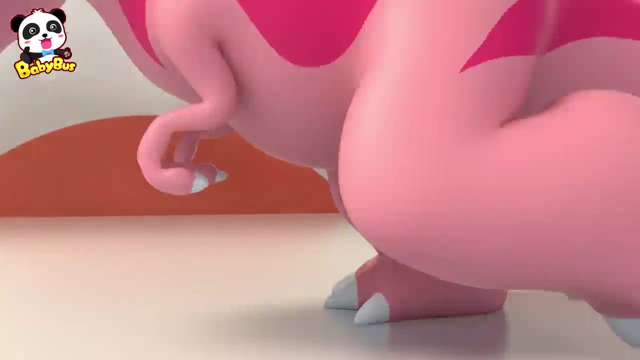 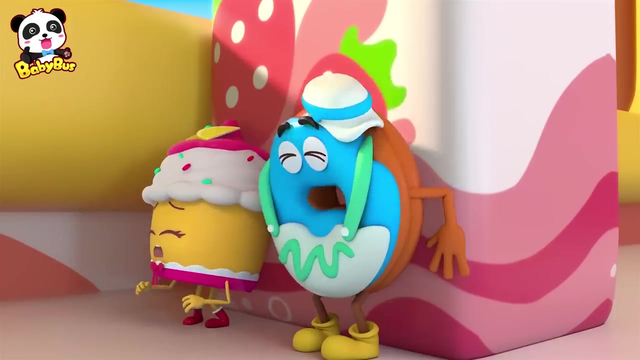 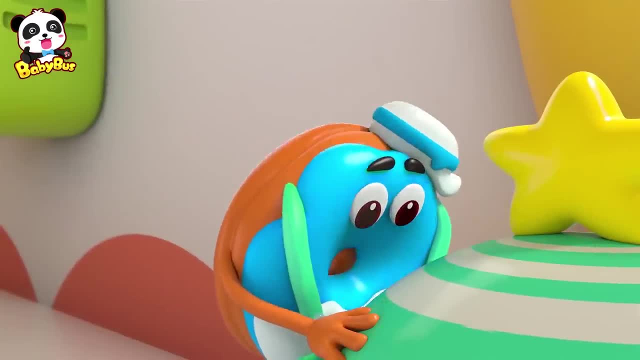 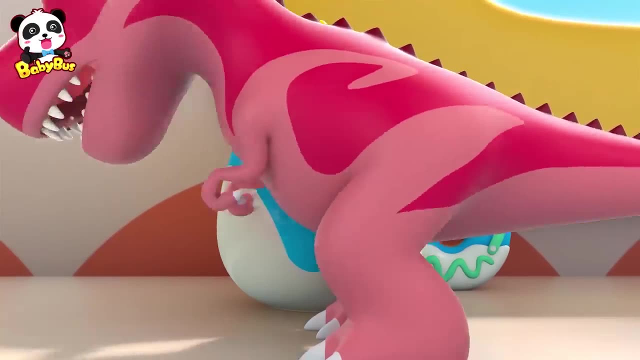 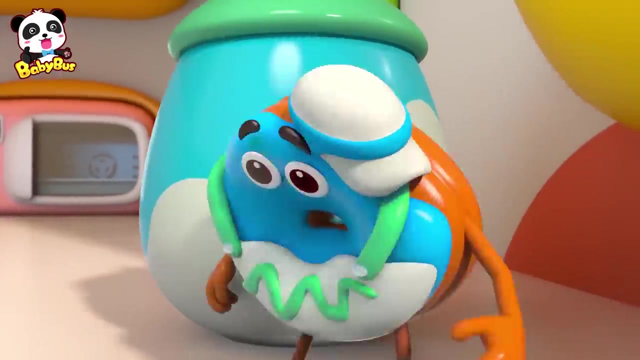 Ha Woo, I have an idea. It's this: Shhh, Stay here and be quiet. Ah, This, Ah, Phew, Phew, It hurts, It hurts, It hurts. Hm Whew, I really did. 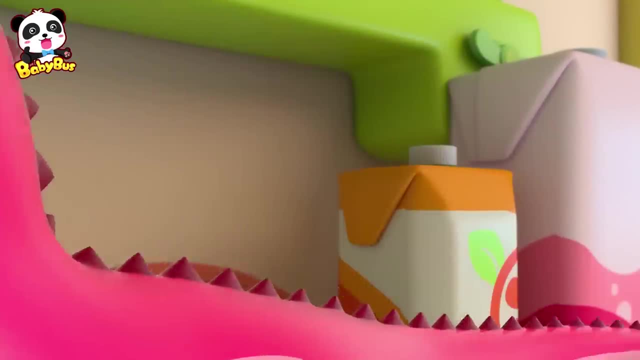 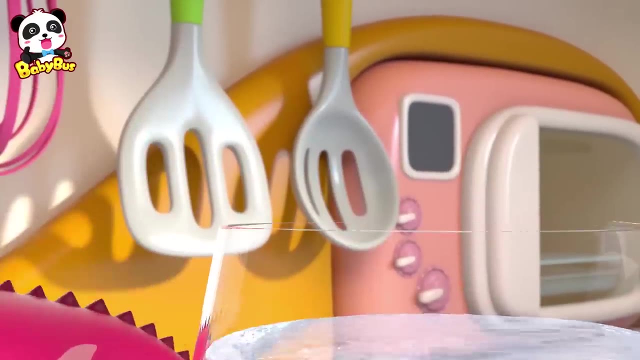 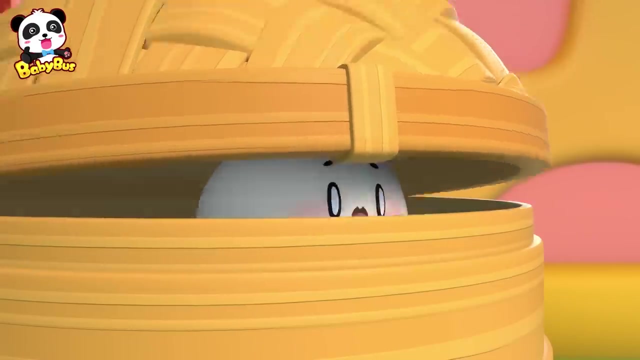 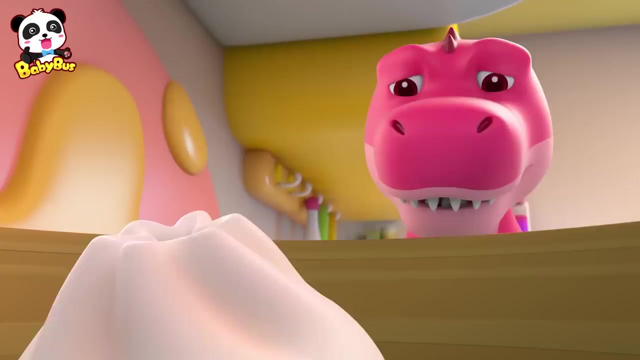 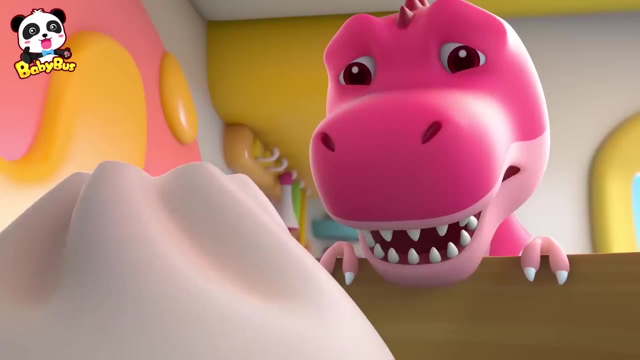 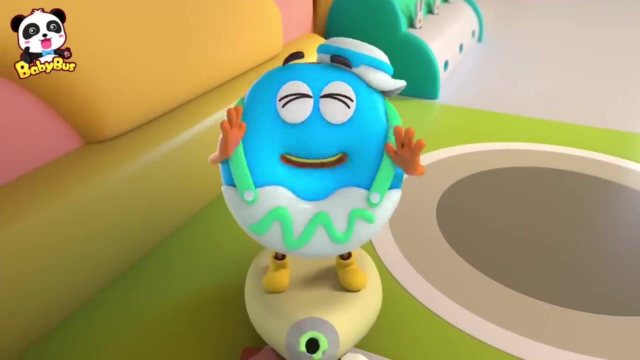 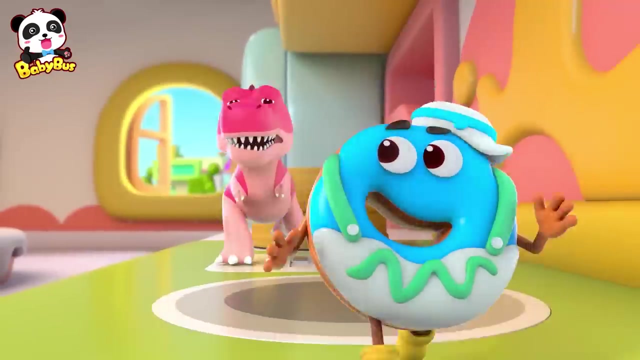 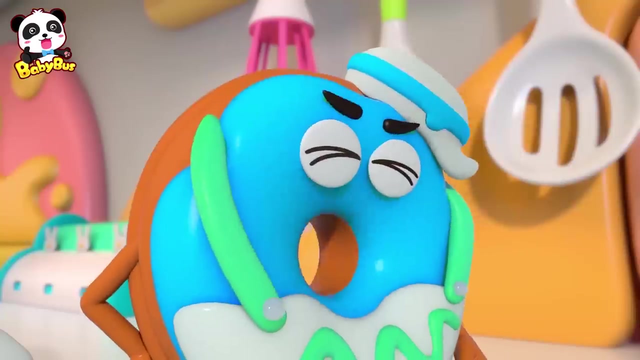 Phew, Whew, I did to you. Phew, Don't hit me. don't hit me, I don't taste very good. Hey, dino, Come and get me, You can't catch me. Ouch, that hurt. 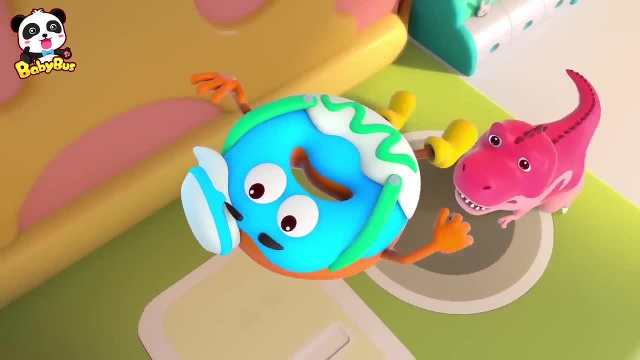 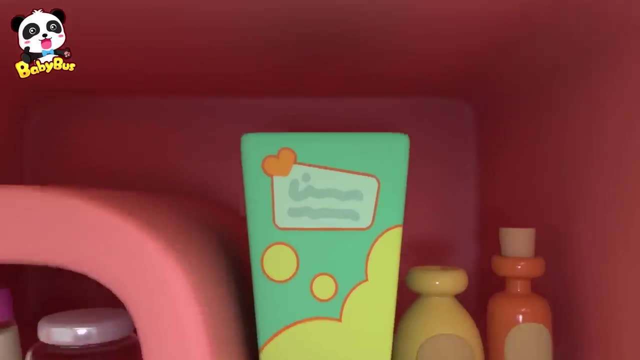 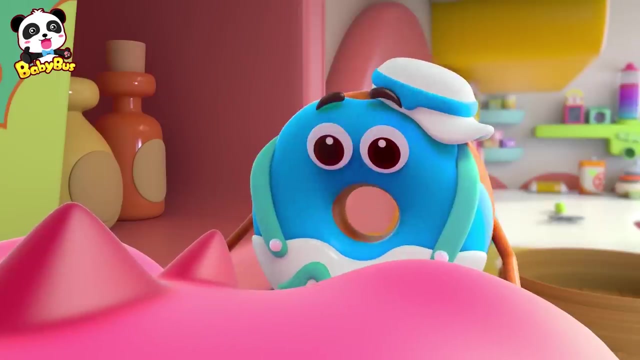 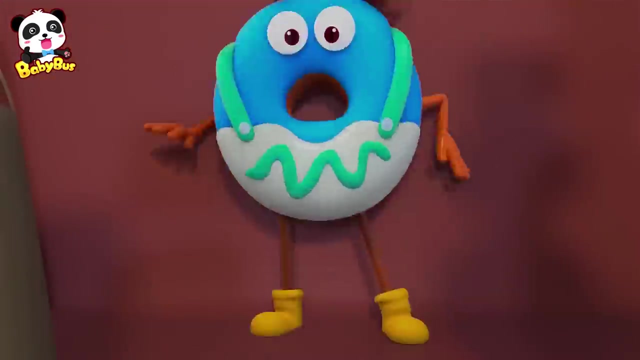 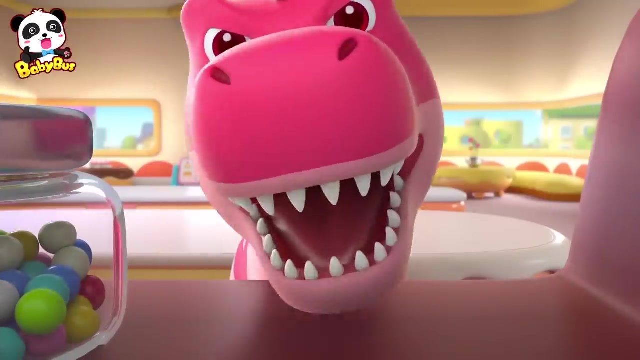 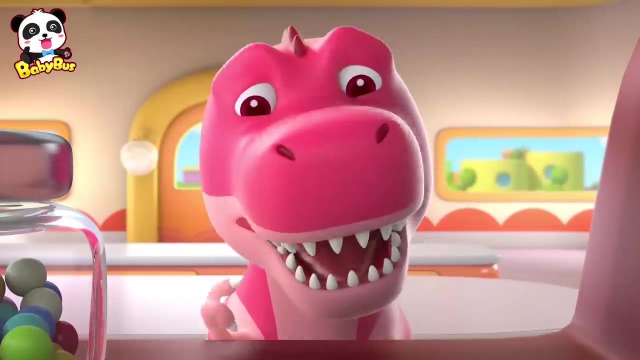 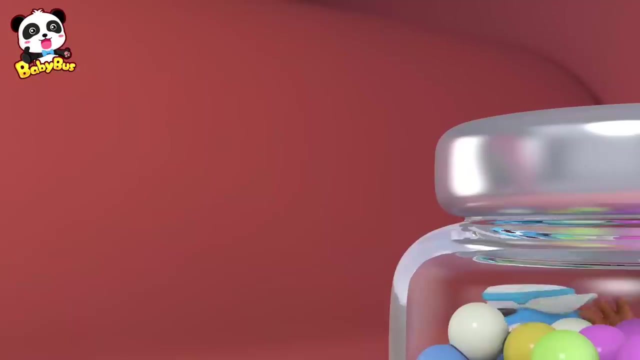 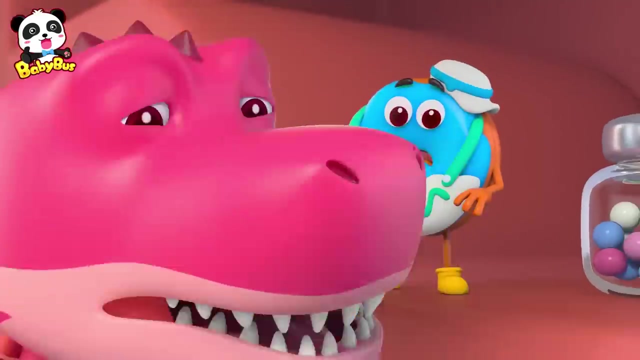 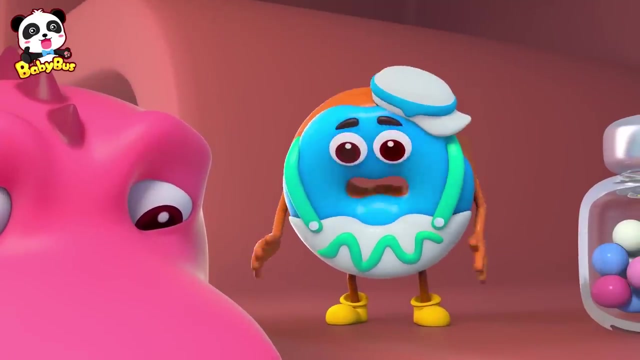 Ouch, Where am I? Wow, it's so high. Don't, Don't eat me, Don't eat me, Let him go. Let him go, you bad dino. Calm down, guys. We misunderstood the dino. 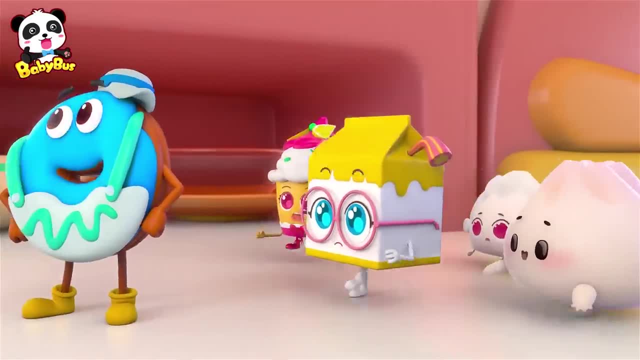 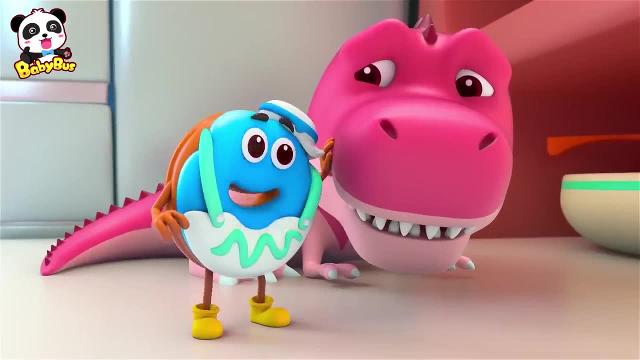 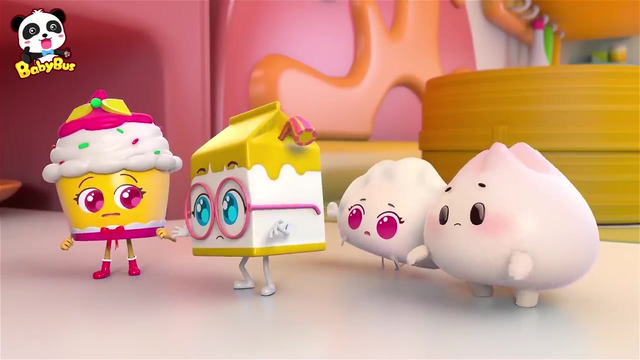 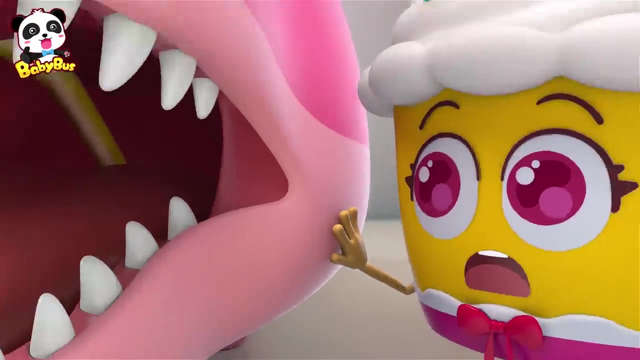 Thank you, dino. Donny, what's going on? We misunderstood him. He wasn't trying to eat us, but asking for help. He needs our help. Look Something stuck in his mouth I see. It must be so painful. 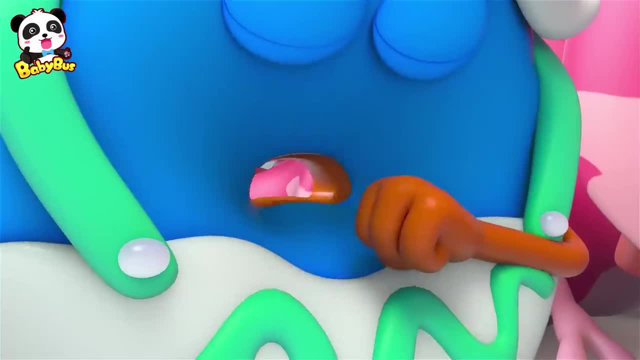 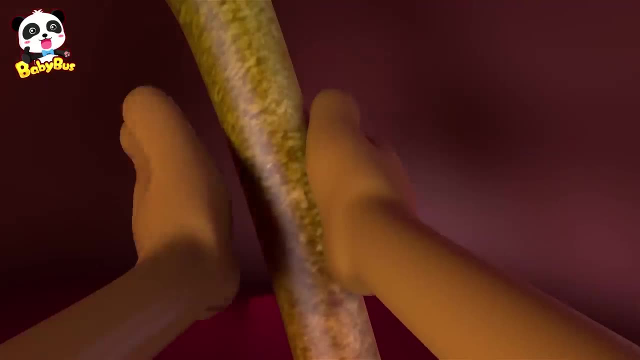 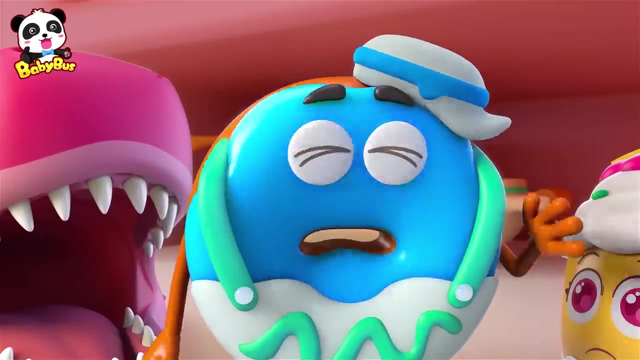 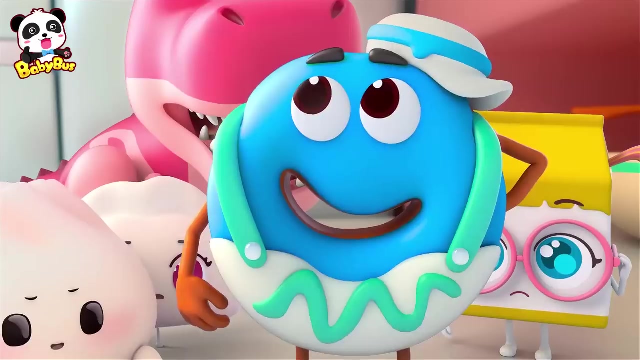 How can we help him? I have an idea. I have an idea. It's so tight. It's so tight I can't pull it out. What should we do, Mom? let's do it together, Together, Aha. 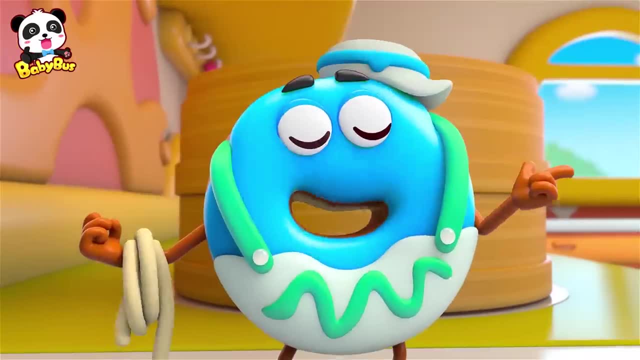 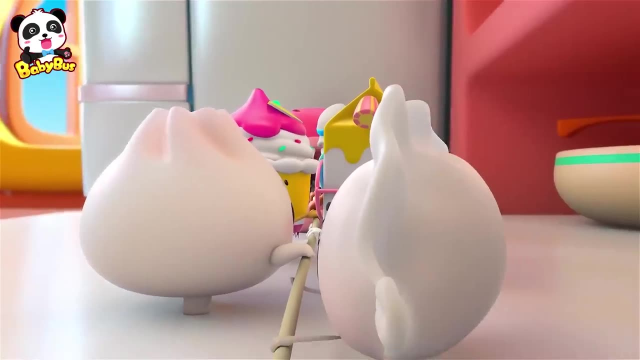 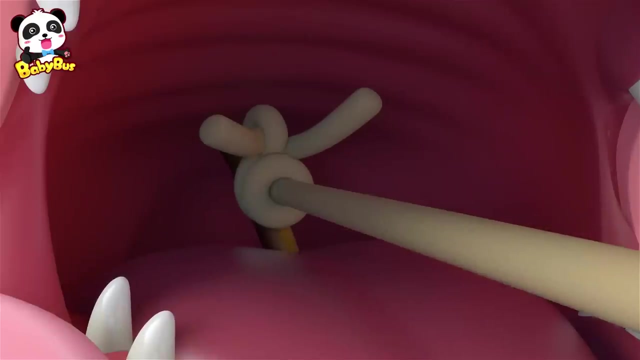 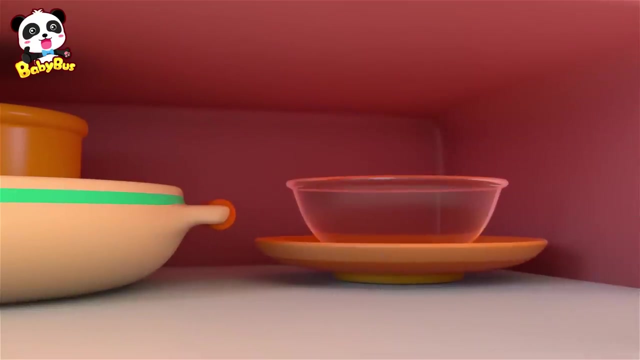 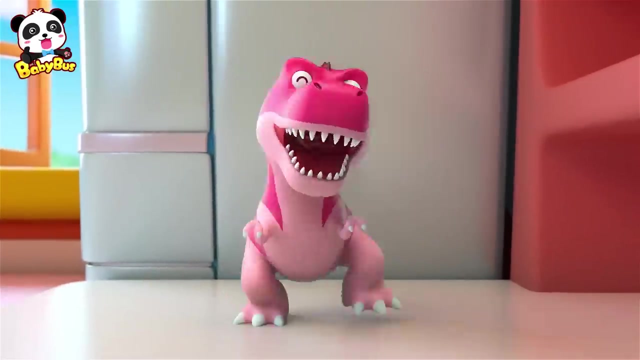 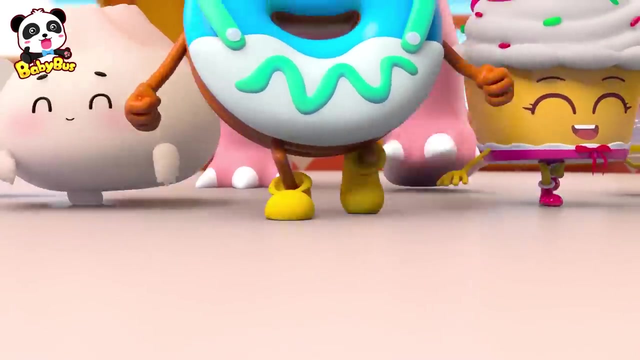 Ta-da, Let's pull it out with this On my mark: One, two, pull, One, two, pull, One, two, pull. Yay, We did it. Here are little friends and a big T-rex. 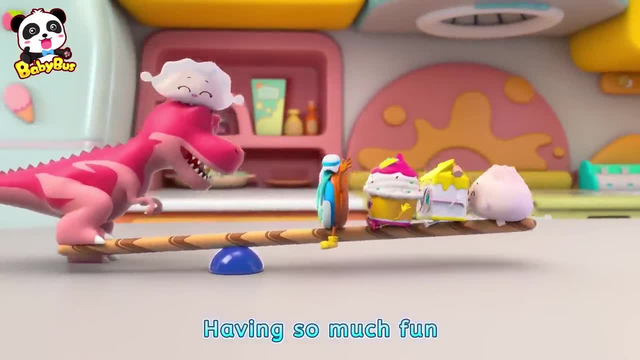 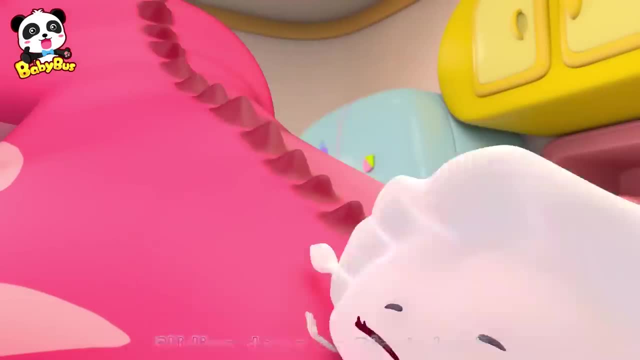 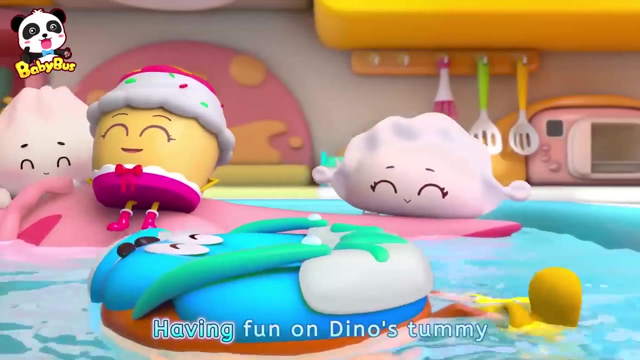 We are all friends now having so much fun. Let's slide down. It's so much fun Sliding down on Dino's back into the water. Let's swim around. It's so much fun Having fun on Dino's tummy. 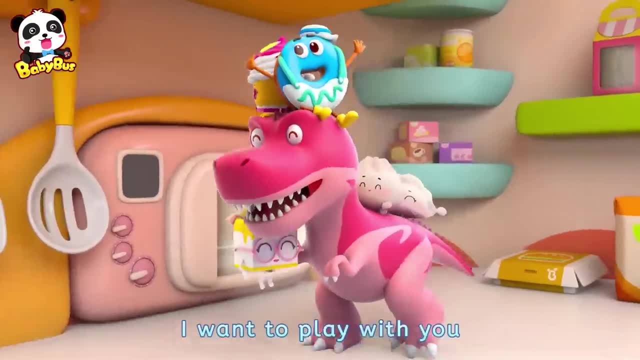 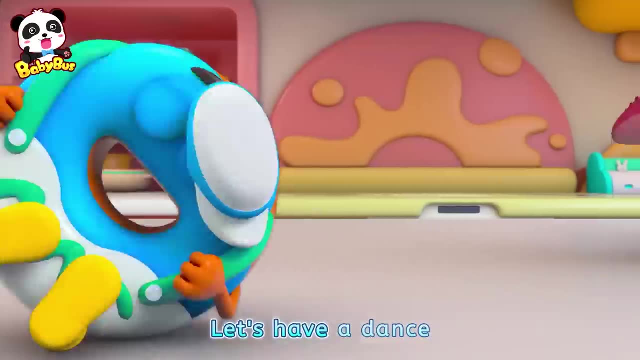 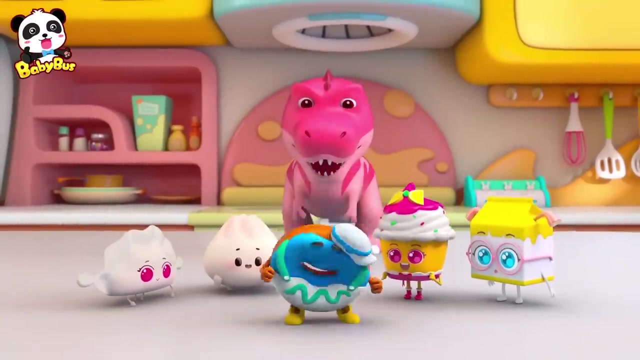 We're happy. Come on, my good friends, I want to play with you. Come on, my good friends, I want to dance with you. Let's have a dance, My friends, let's have a dance. Your cake was really yummy. 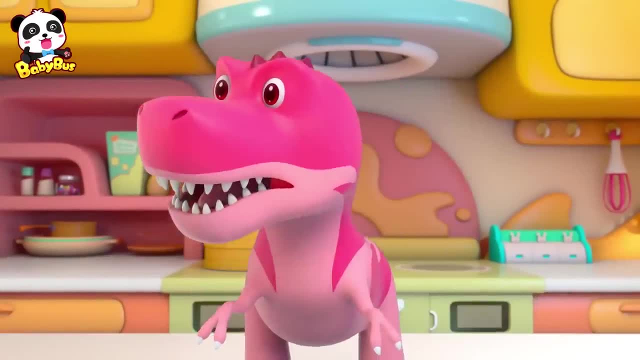 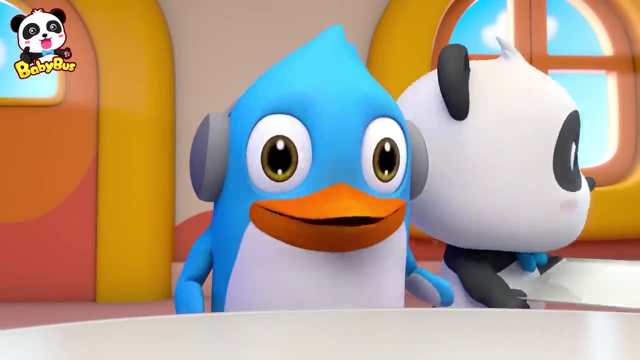 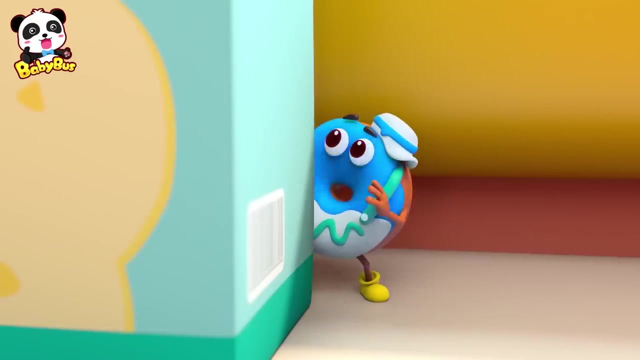 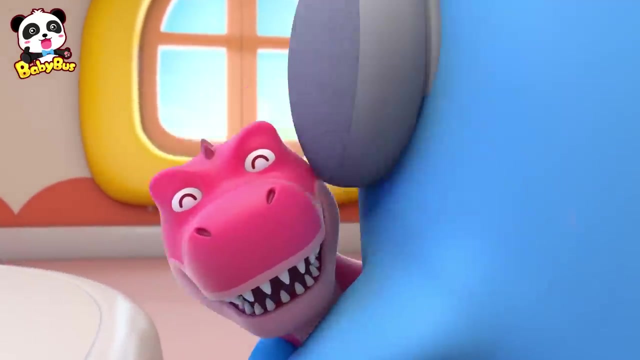 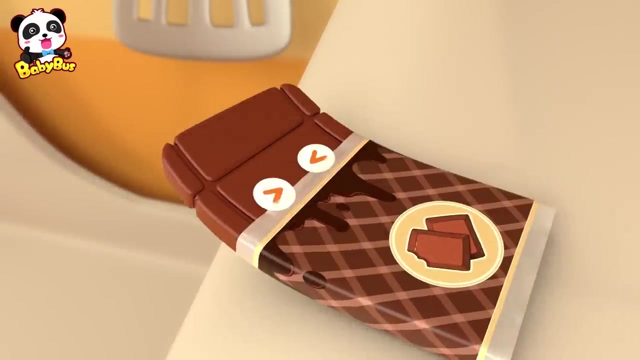 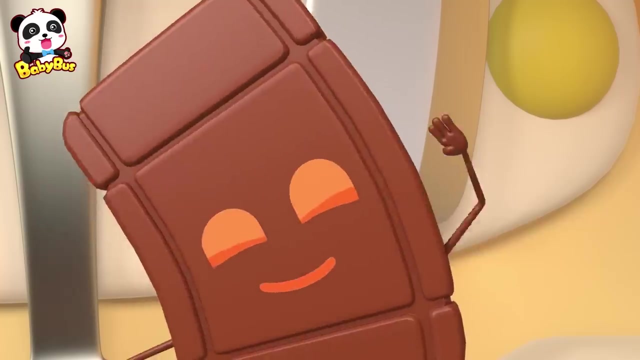 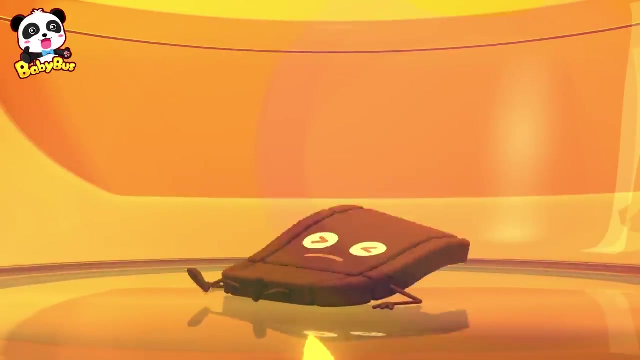 They're coming back. Hi everyone, My T-rex, Let's go home, Let's go home. He's going home. He's going home. Bye, Dino, Bye. Oh, that hurts. Hey, where am I? Huh? 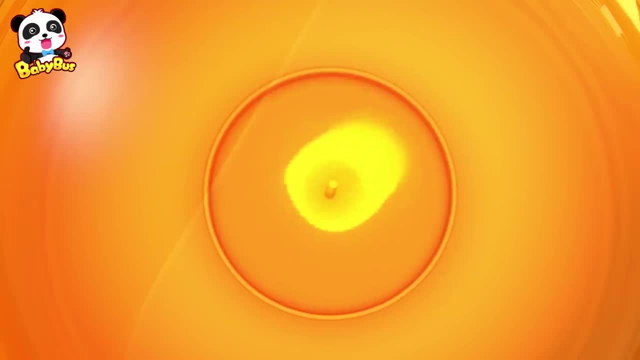 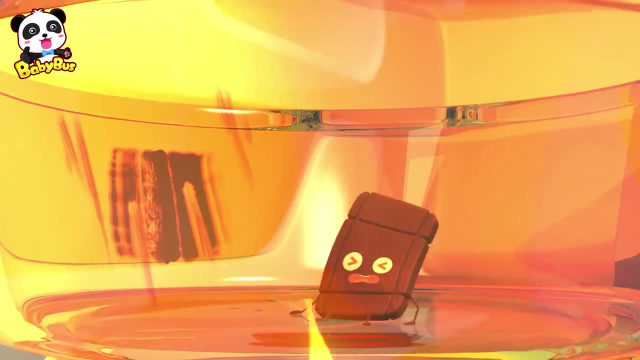 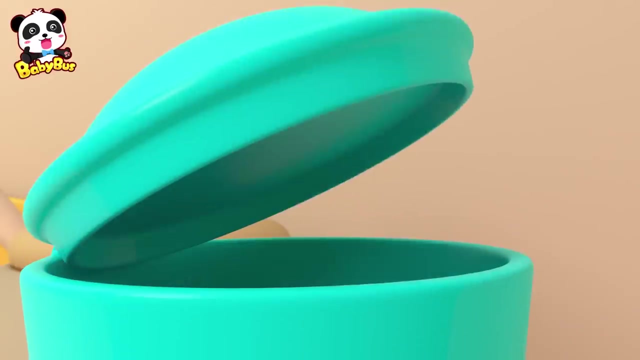 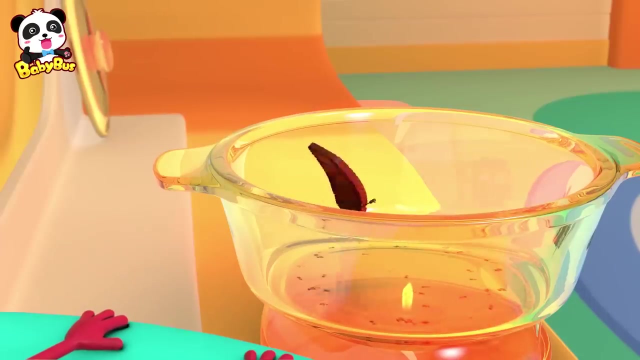 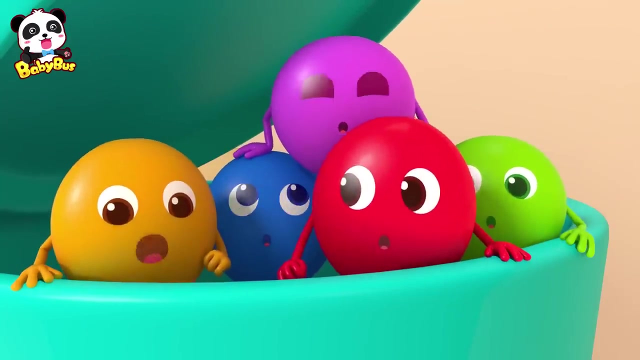 Huh, Oh, Help, Help, Let me out. Help, Someone help me, Help. Huh, What's going on? Help, I'm melting. It's chocolate. He's in trouble. Let's help him. We have to put the flames out. 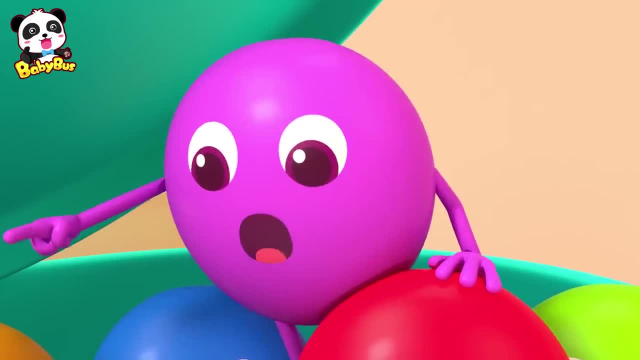 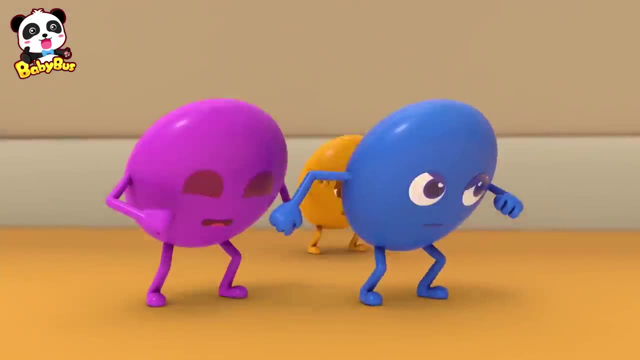 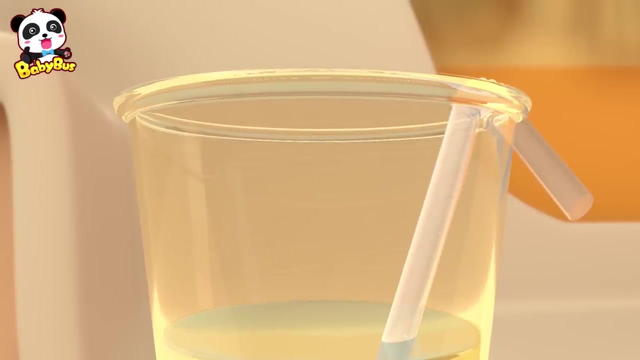 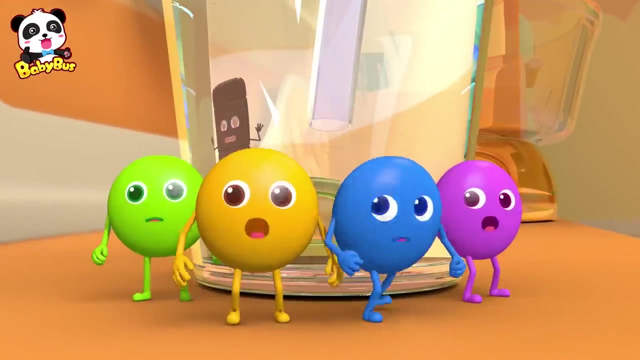 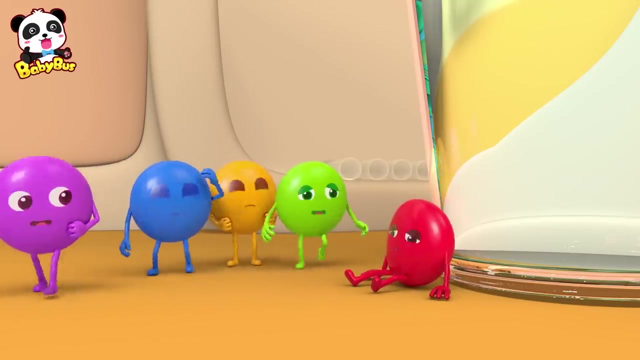 The flames. Look, We can use water to put the flames out. We can use water to put the flames out. We can use water to put the flames out. Watch me, It didn't move at all. What should we do? We're not strong enough. 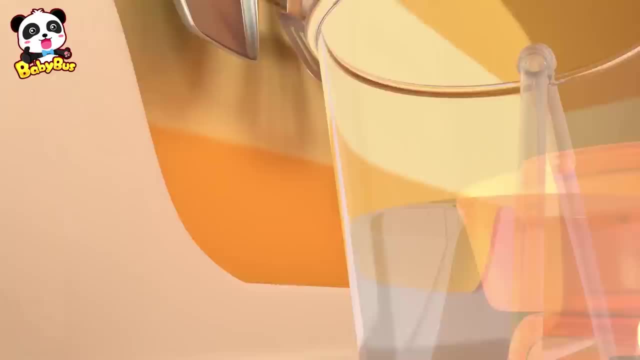 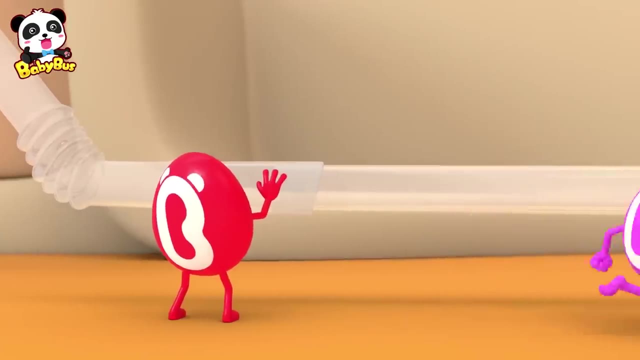 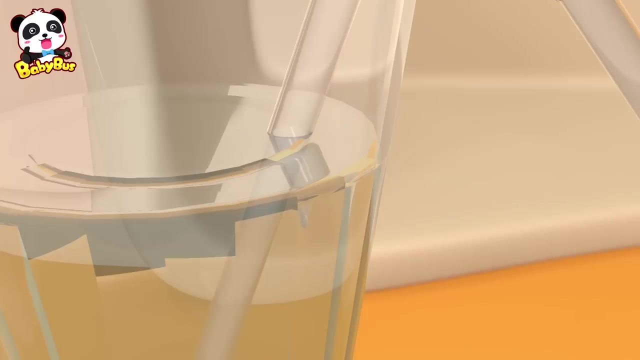 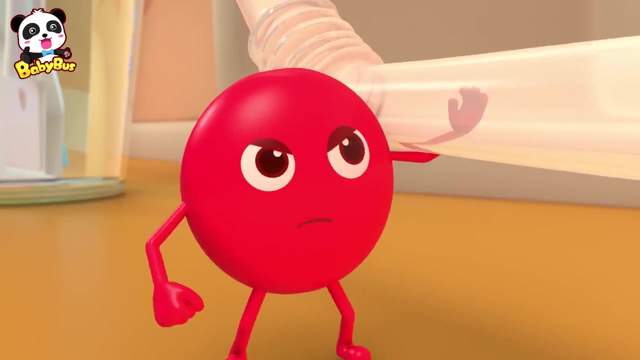 Hmm, I got an idea. I got an idea. Come with me. Huh, Huh, Huh, Help, Help me, I'm melting, I'm melting. Help, Hold on, We're coming to help you. We're coming to help you. 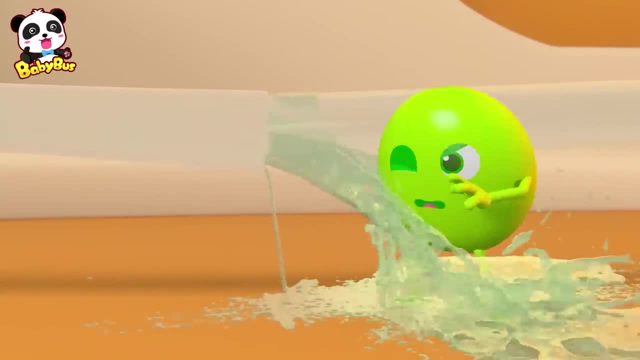 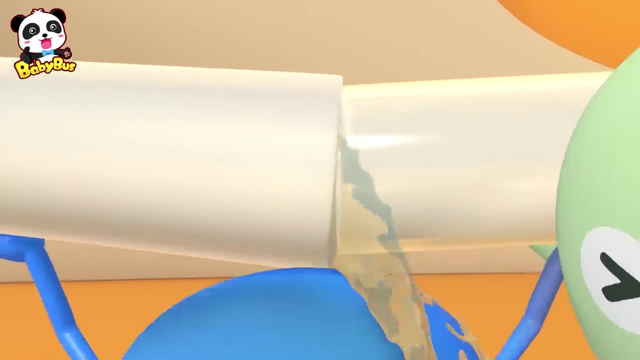 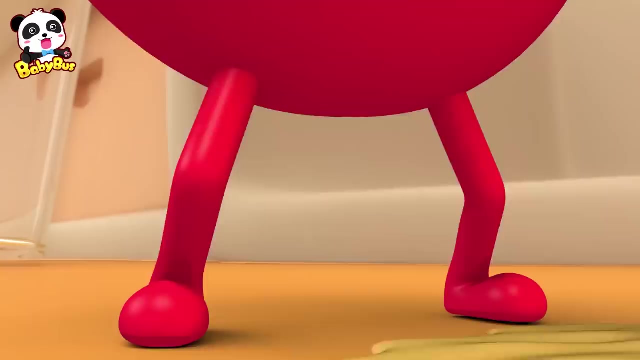 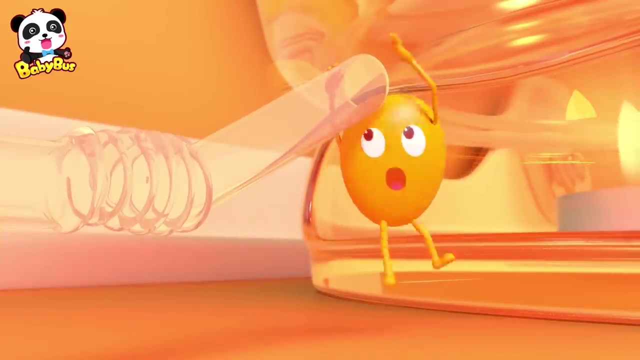 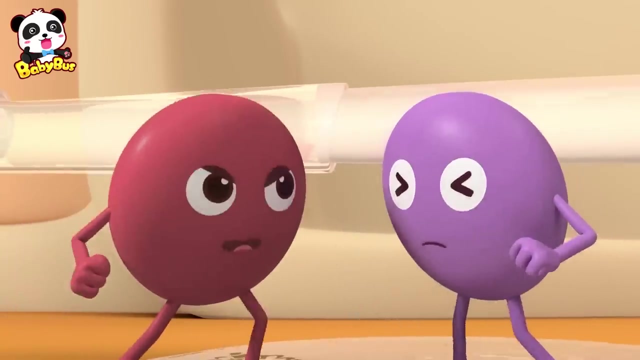 We're coming to help you Help. Oh no, The water is coming out. Let me help you, Help, Help, Help. Great job, Help, Help. Oh no, I'm coming, Help, Help, It's fixed. 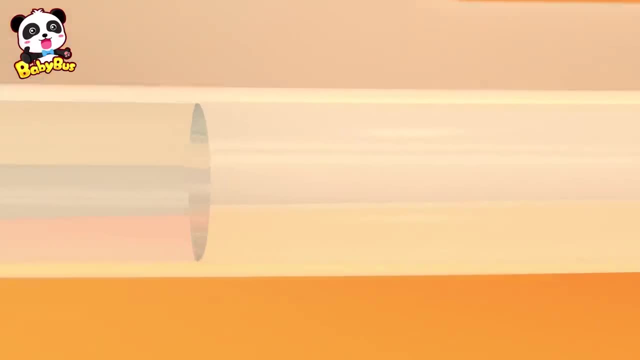 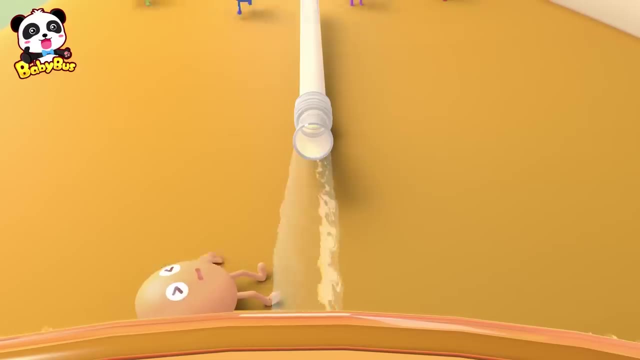 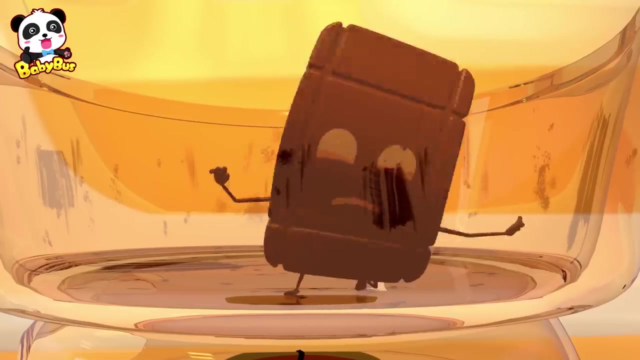 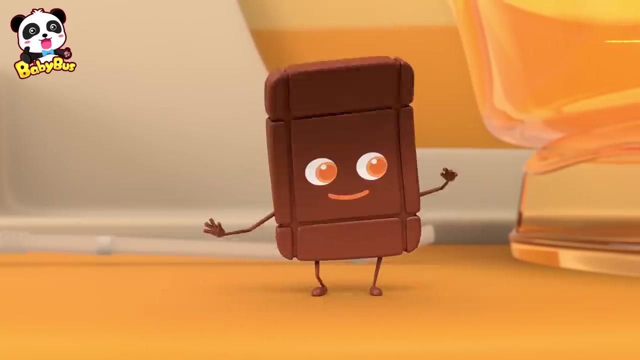 Let's save chocolate. OK, Let's save chocolate, Let's save chocolate. Yay, Yay, Help, Help, Help. Yeah, I'm saved, I'm saved. Phew, I almost turned into chocolate sauce, Thank you. 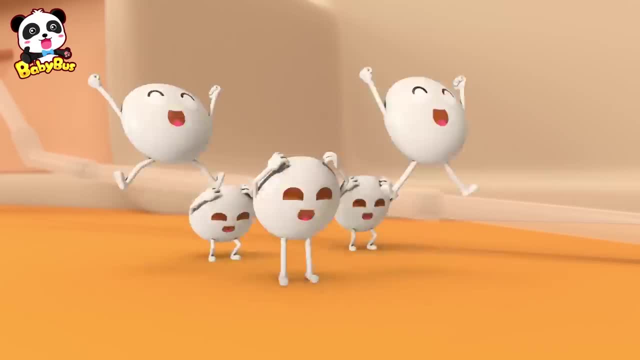 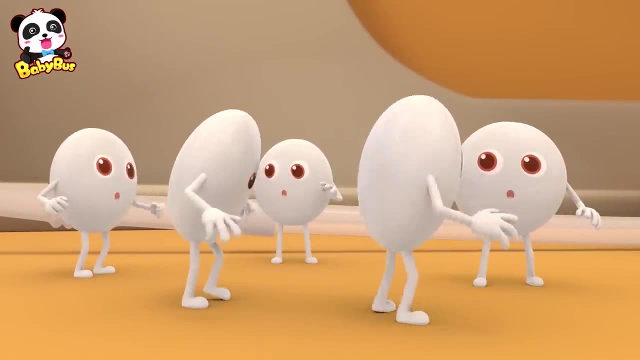 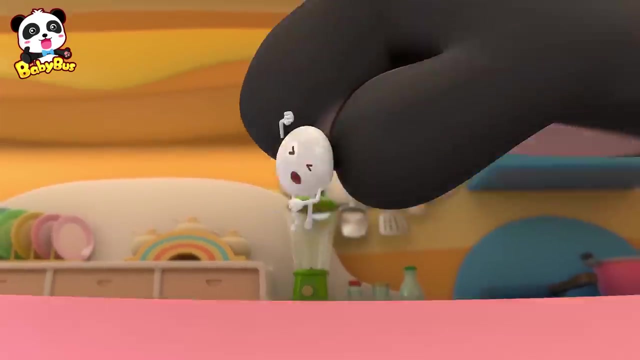 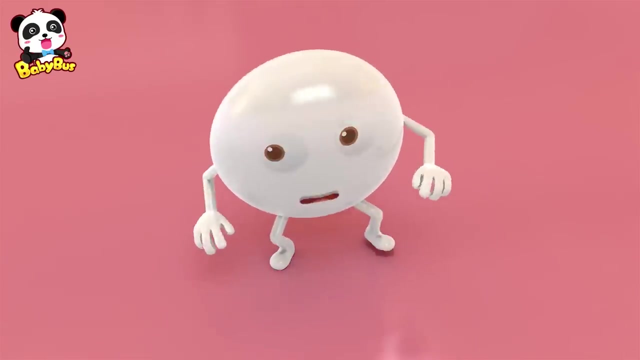 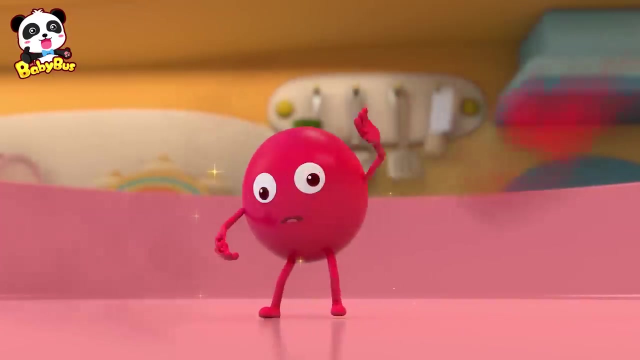 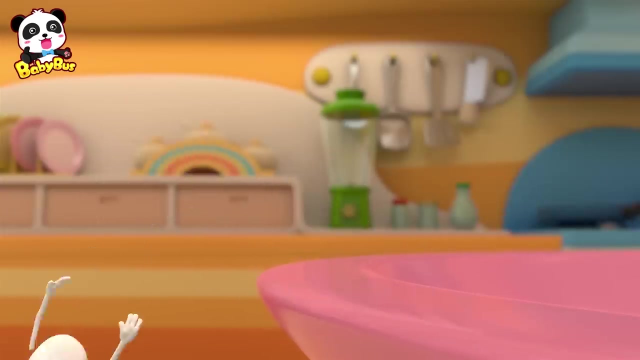 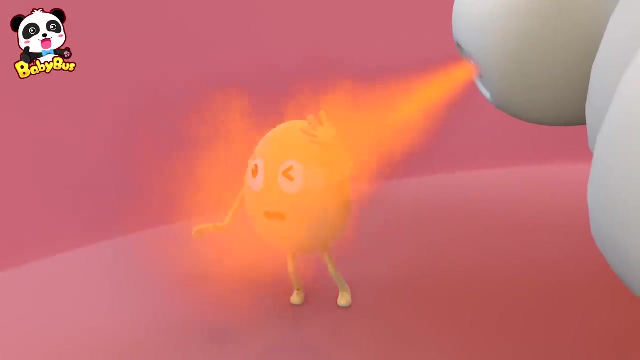 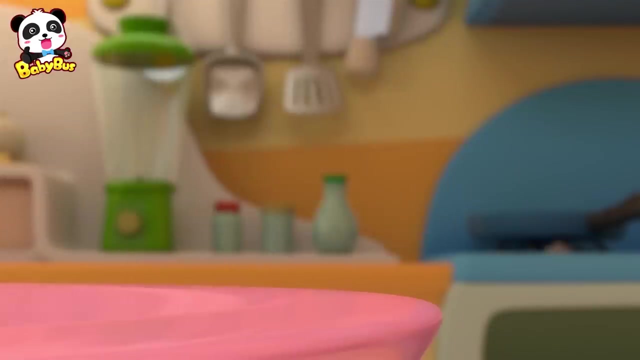 Uh, who are you? We're going for candy. Where are your colors? Huh, What happened? Whoa, Run away, everybody, Run away, Run away Red. Huh, I'm yellow. Oh, Oh, Oh. 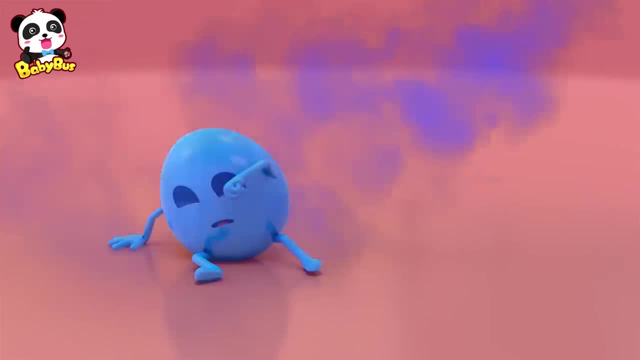 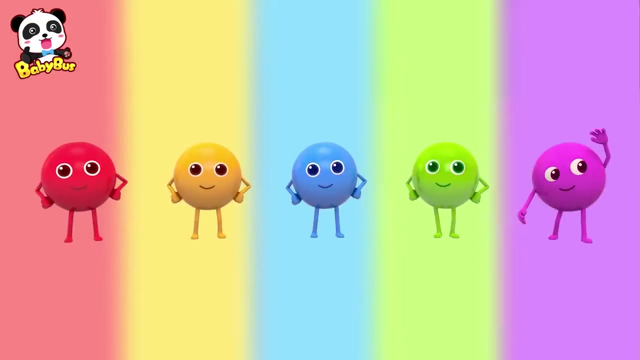 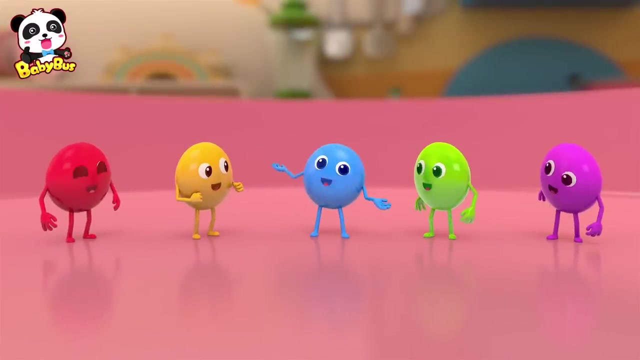 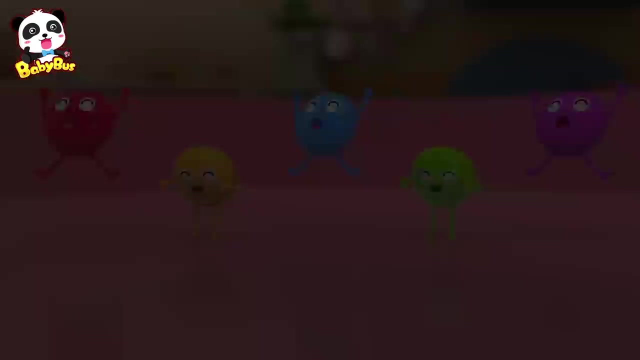 Oh, Oh, Huh, Blue, Huh, Green, Ah, Purple, Red, Yellow, Blue, Green And purple. So Kiki tried to put colorful clothes on us. Ooh, Thank you, Kiki, I'm so excited. 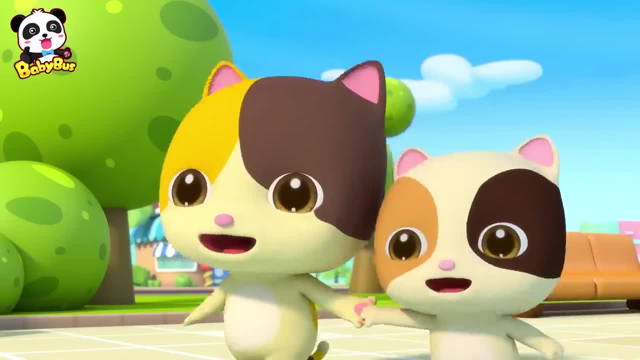 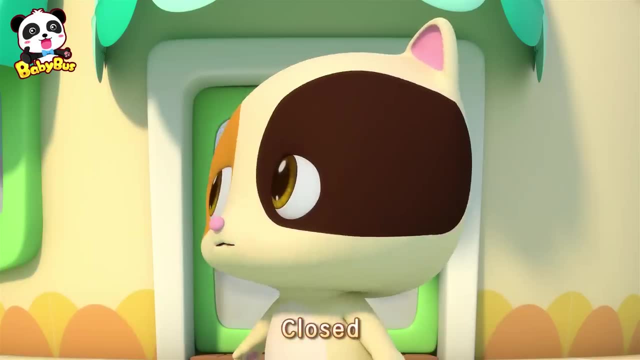 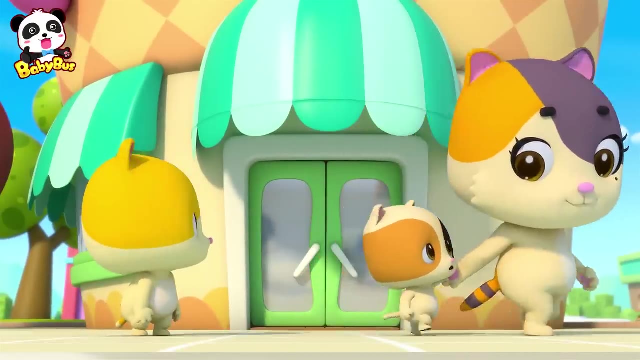 Which ice cream should I pick? La-la-la-la-la, Huh Huh. The ice cream shop is closed today, Closed, Ooh. Well, then let's come again tomorrow. Ugh, Look, There's an ice cream vending machine. 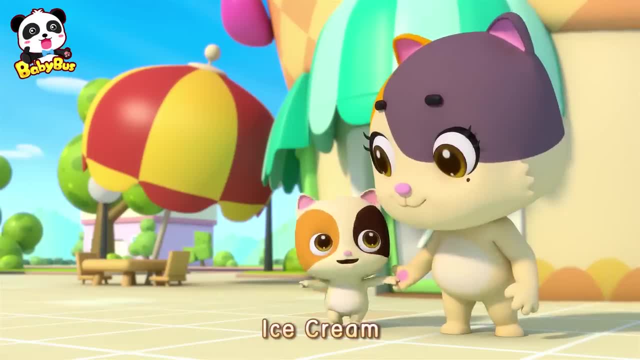 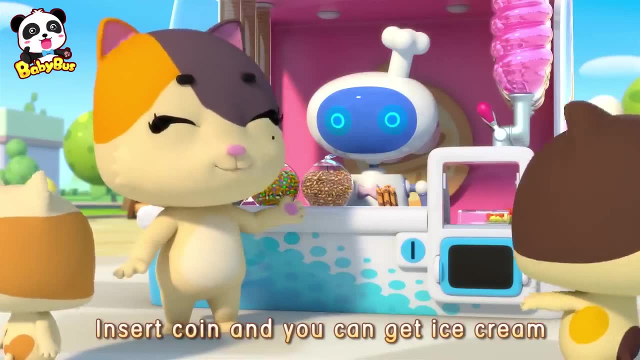 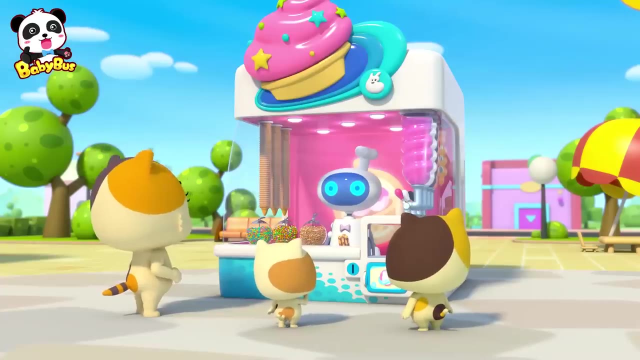 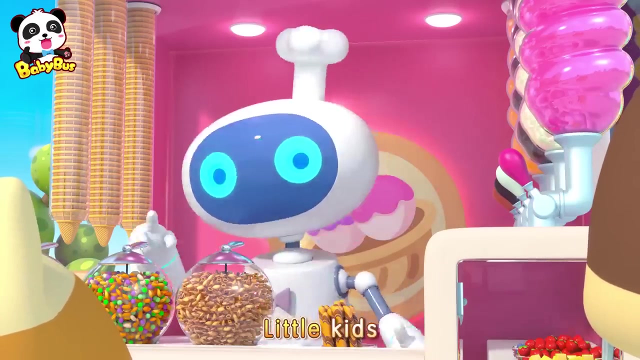 Huh, Ice-cream, Ice-cream. Mom, I want ice-cream. OK, OK, Insert coin and you can get ice cream. Uh, Ice-cream, Slurp. Robot vending machine selling yummy ice cream. Come and see, little kids, many flavors you can choose. 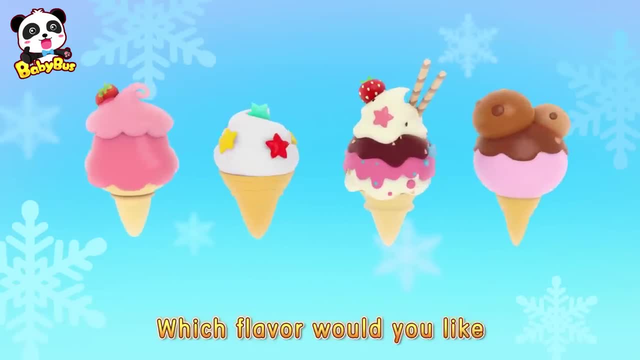 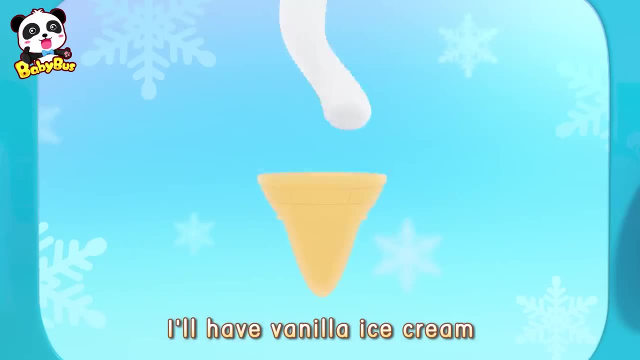 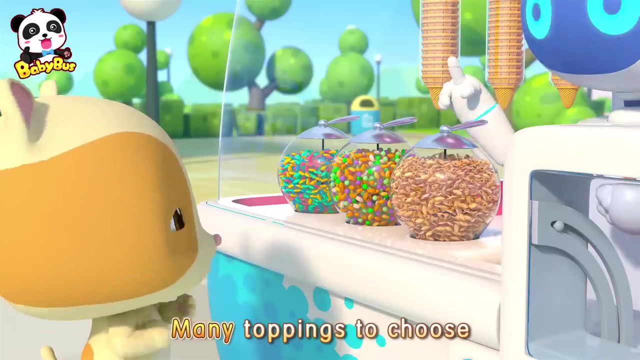 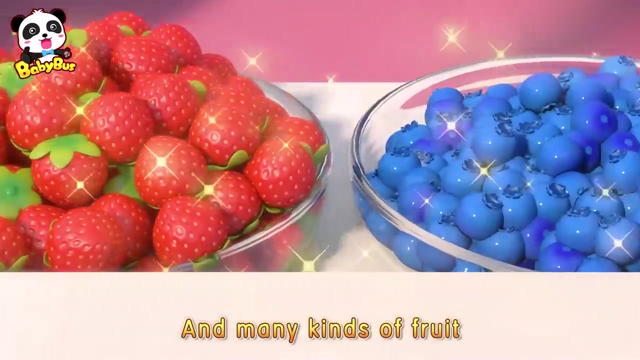 Strawberry, chocolate, vanilla. which flavor would you like? Let me think about it. I'll have vanilla ice cream. Robot vending machine selling yummy ice cream. Many toppings to choose: rainbow colored candy, Many kinds of nuts and many kinds of fruit. Which topping would you like? 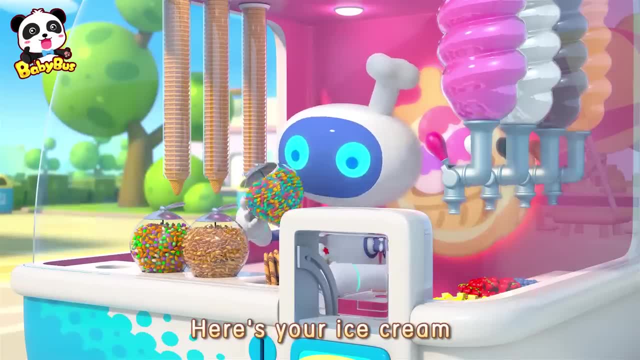 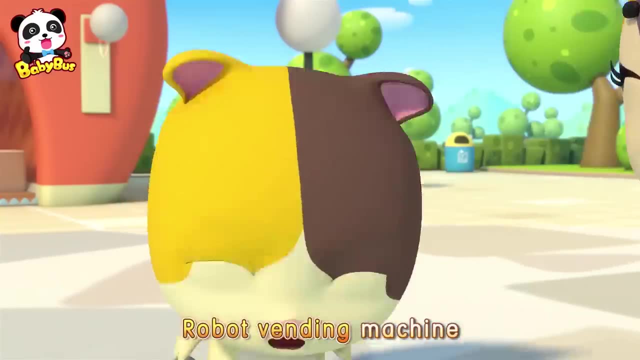 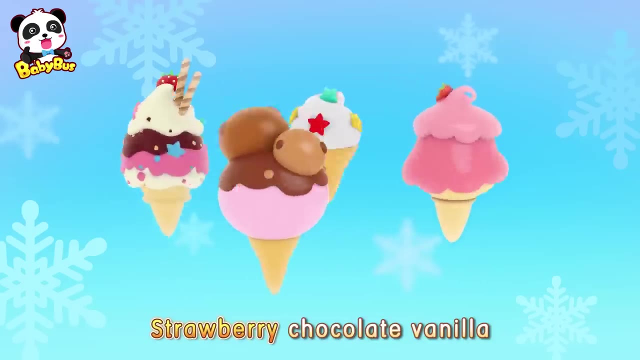 I'll have the rainbow colored candy. Here's your ice cream. enjoy Mom. a coin, a coin, please. Robot vending machine selling yummy ice cream. Come and see little kids. many flavors you can choose: Strawberry, chocolate, vanilla. which flavor would you like? 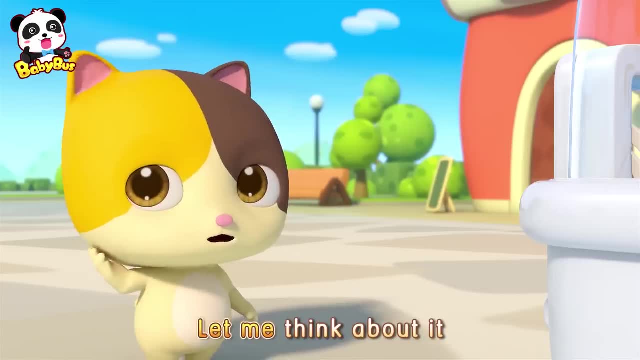 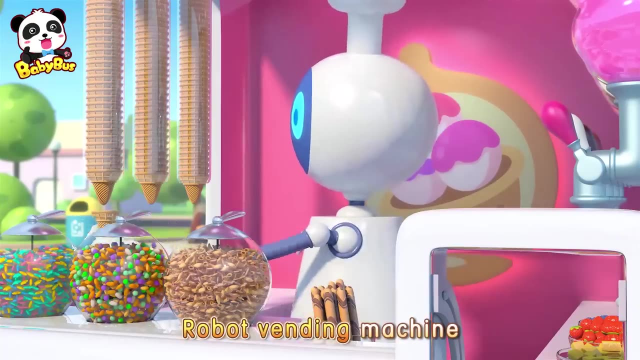 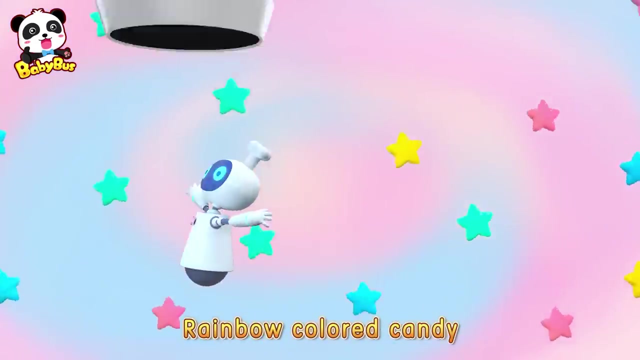 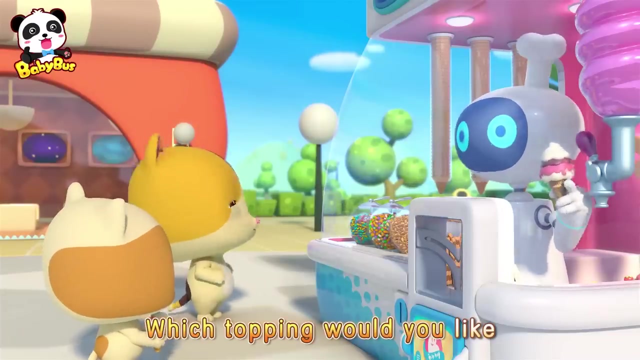 Let me think about it. All flavors, Robot vending machine selling yummy ice cream. Many toppings to choose: rainbow colored candy, Many kinds of nuts and many kinds of fruit. Which topping would you like? I'll have everything. Here's your ice cream with the rainbow colored candy. 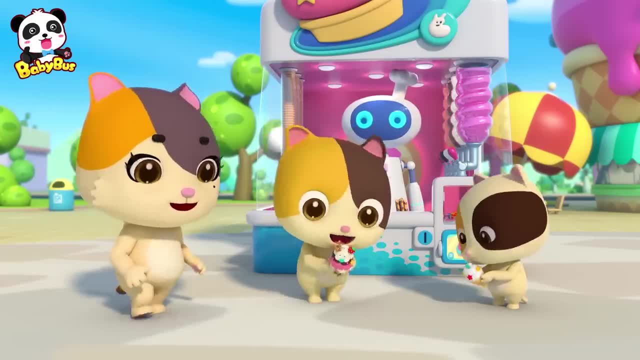 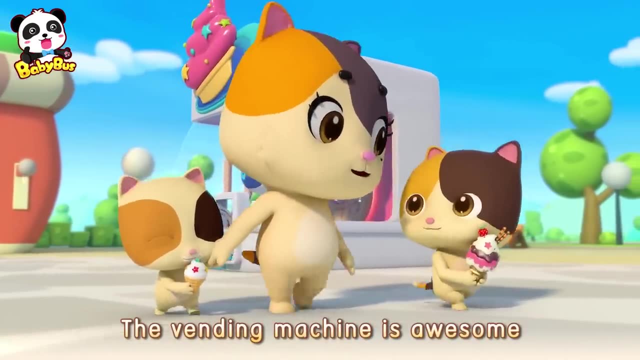 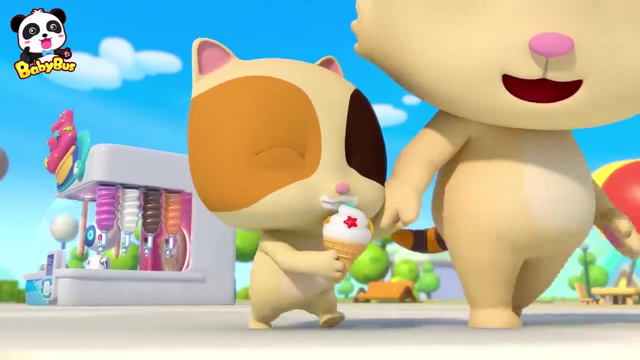 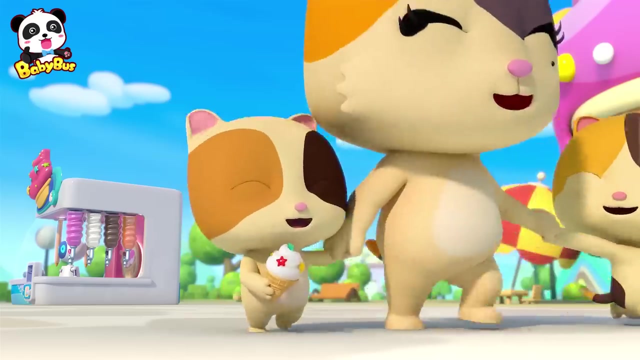 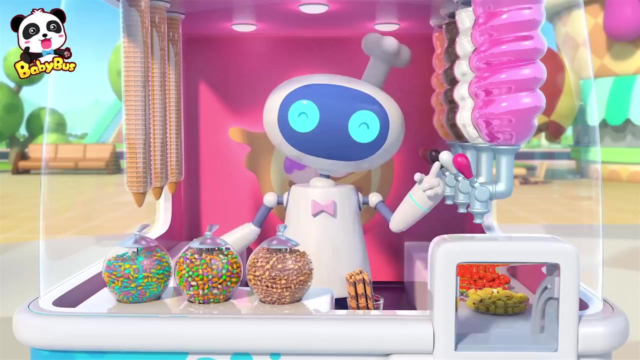 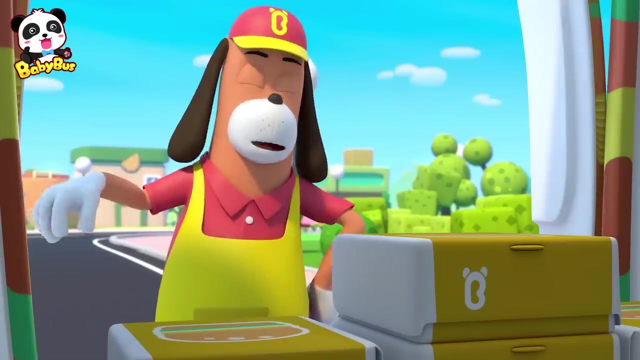 Everything on it. enjoy, Mom. the vending machine is awesome, Right, and it was so fun to use. Look at you: the ice cream is all over your face. Come and see little kids. which flavor would you like? Here's your ice cream with the rainbow colored candy. 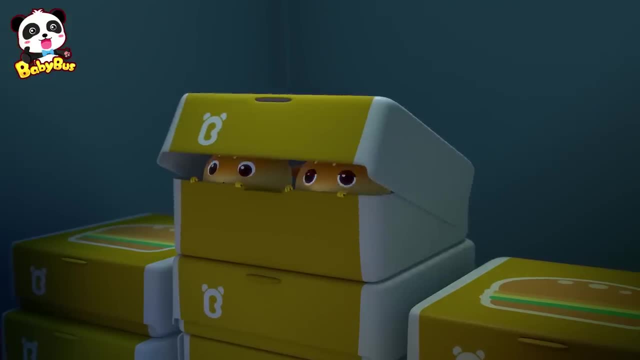 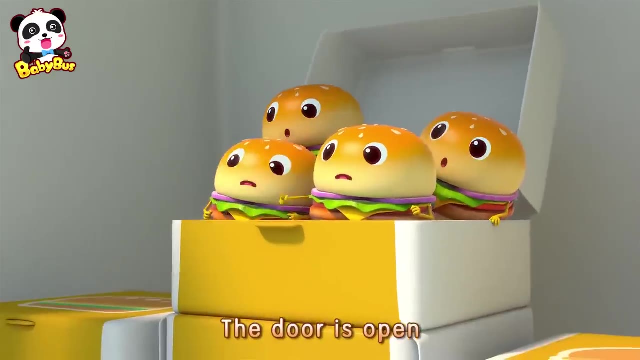 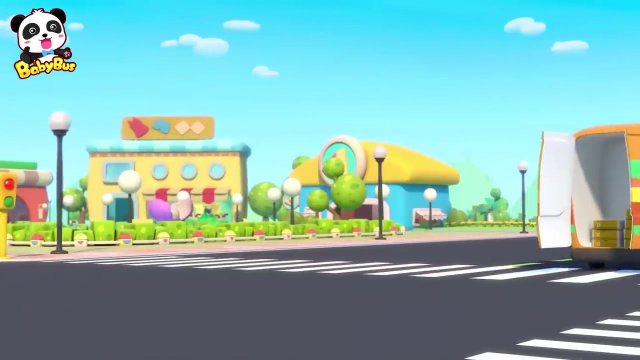 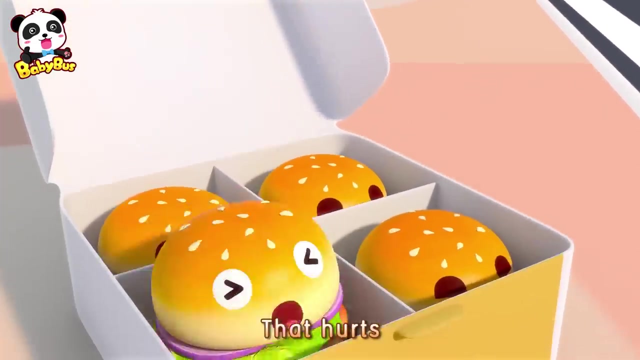 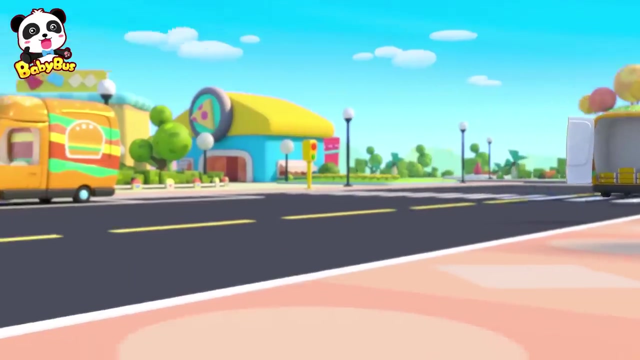 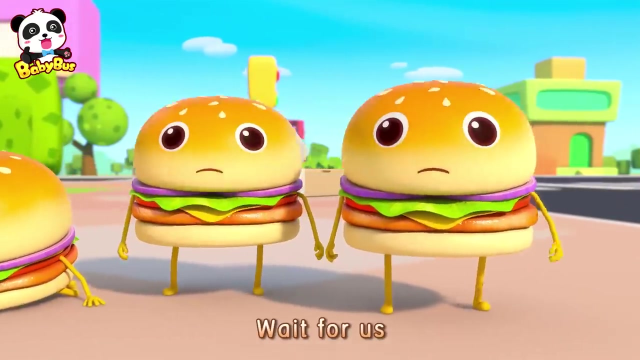 All flavors, all flavors, Let's go get it. Here's your ice cream, let me try. Here's your ice cream, let me try. That hurts The truck. Hey, Hey, What should we do, Truck? Oh no, Wait for us. 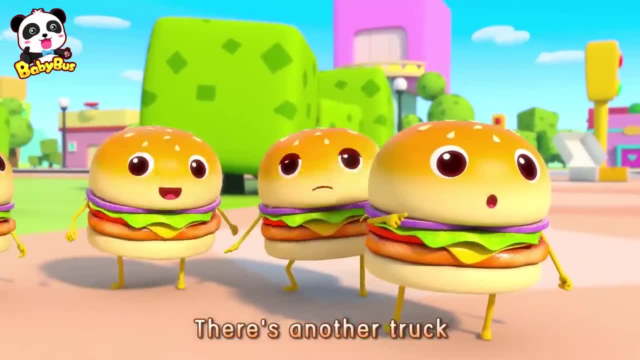 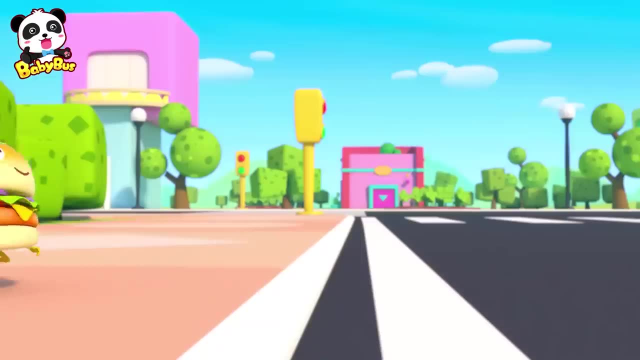 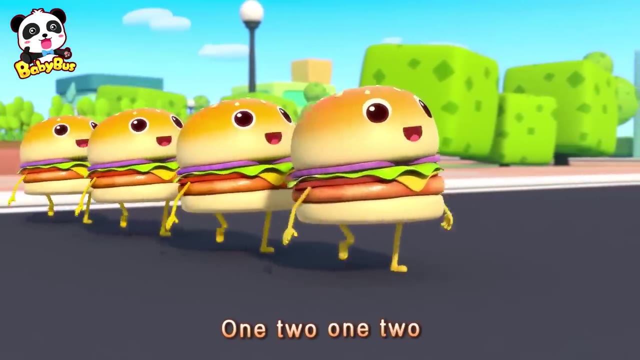 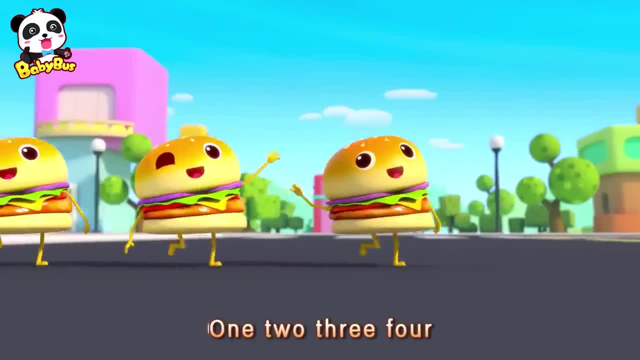 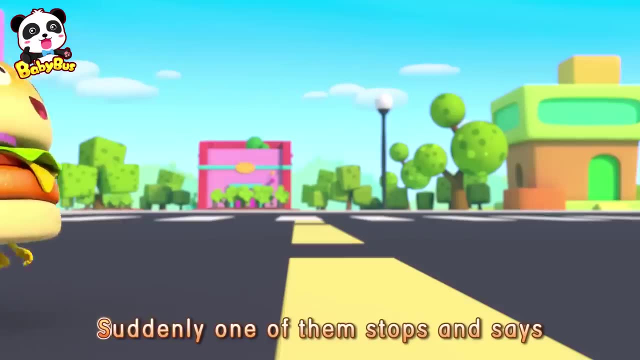 One, two, one, two. March. One, two, three, four, four Little hamburgers- One, two, one, two- Marching on the street. Suddenly one of them stops and says: What is that? What is that? Watch out everyone. 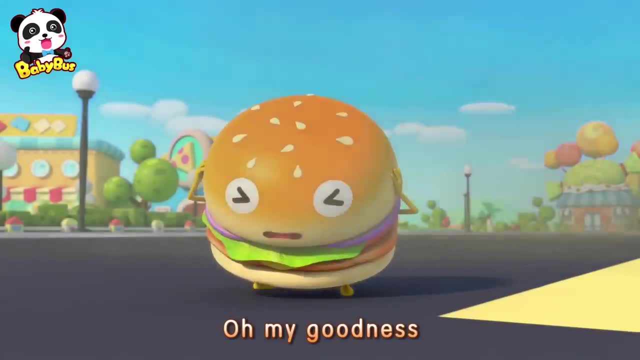 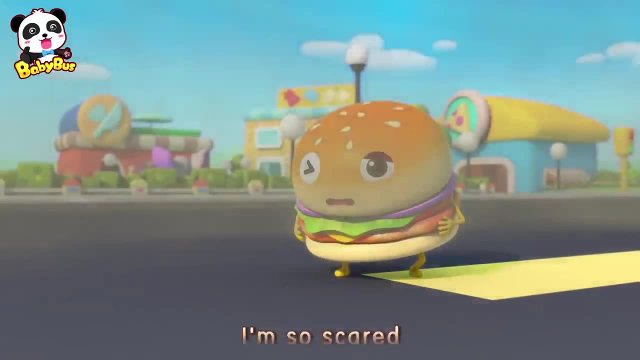 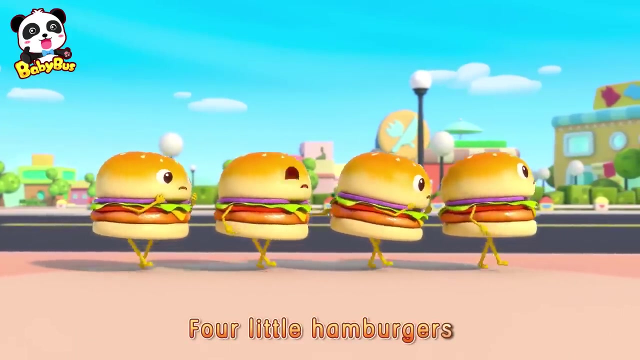 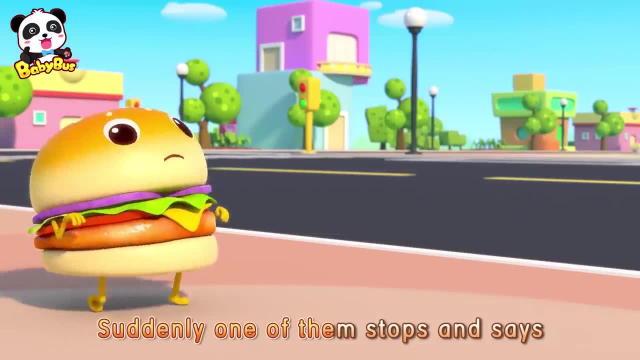 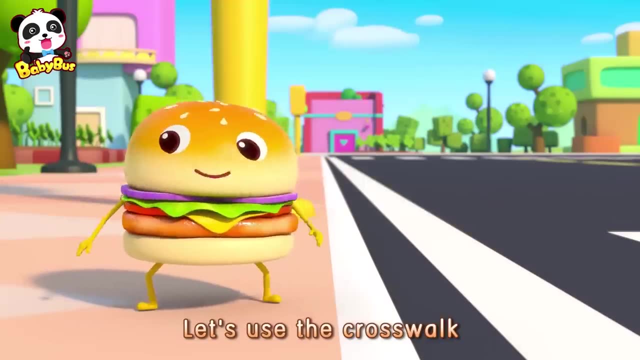 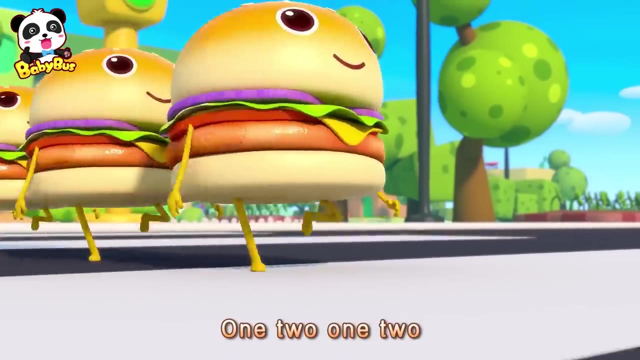 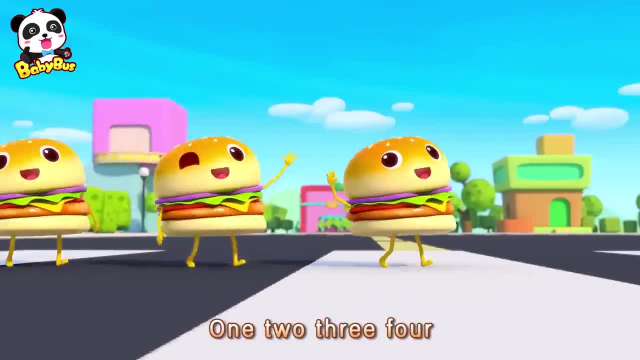 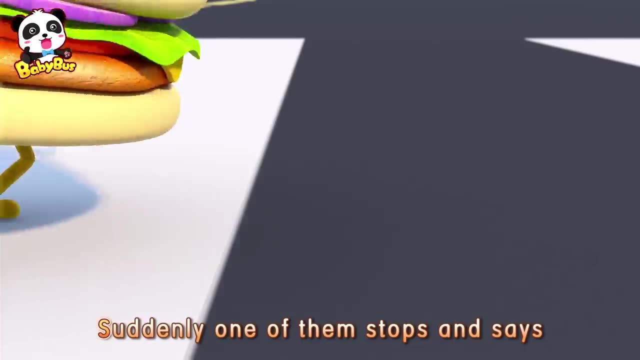 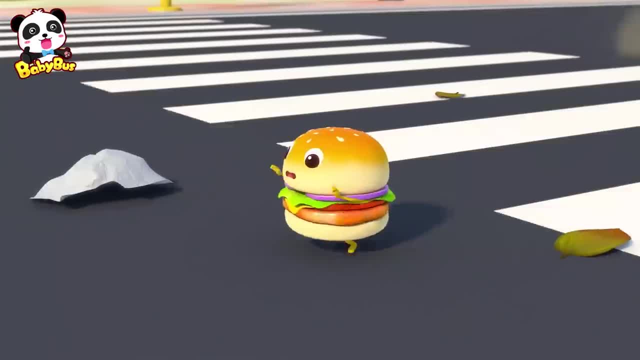 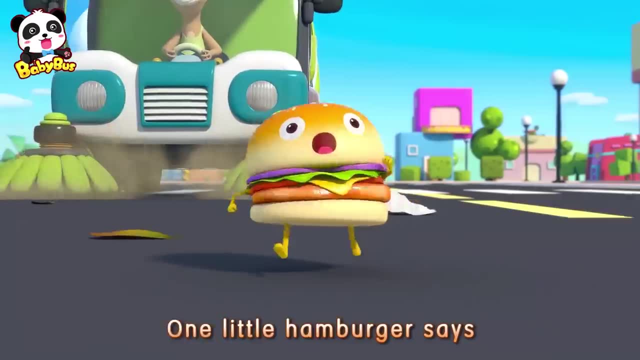 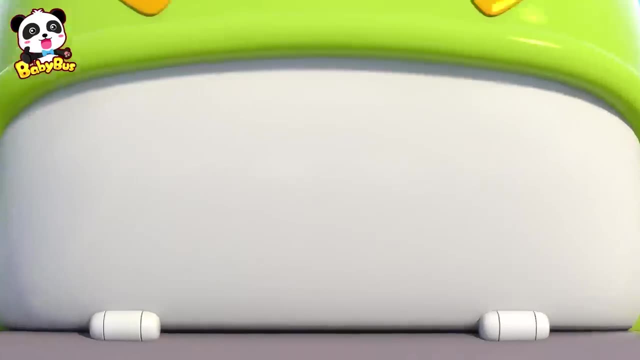 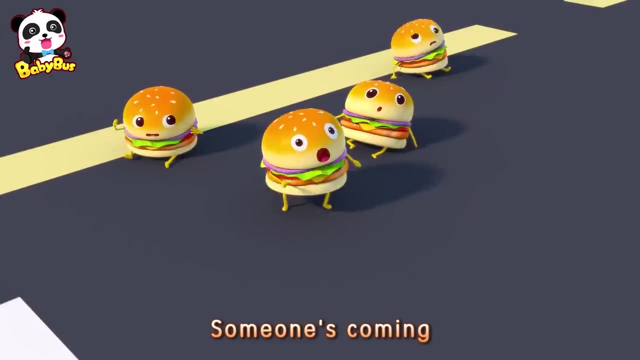 One little hamburger says: Oh my goodness. One little hamburger says: Help me. One little hamburger says: I'm so scared. One little hamburger says: Run away, Someone's coming, Someone's coming. Mr Doll said one box of hamburgers was missing. 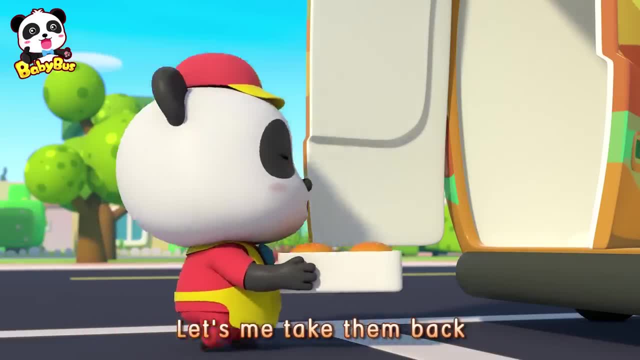 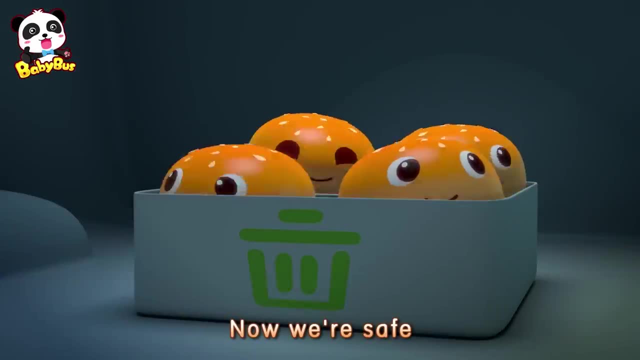 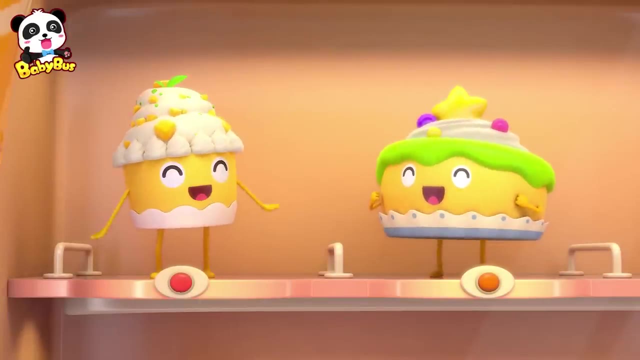 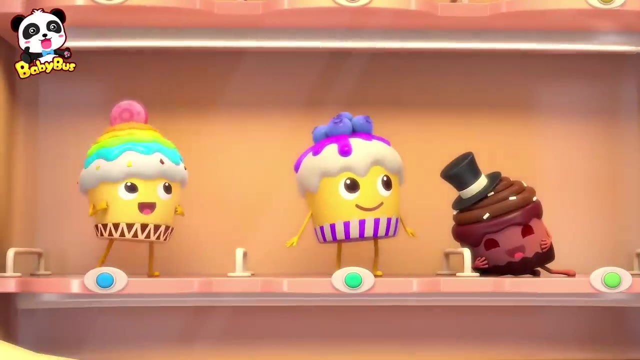 and I think this is it. Let me take them back Now. we're safe. If we're chosen, we'll get to ride down the slide. Yeah, I want to ride the slide, Me too. Me too, Someone's coming. 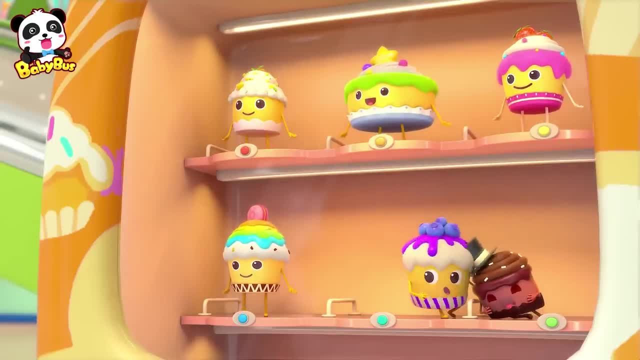 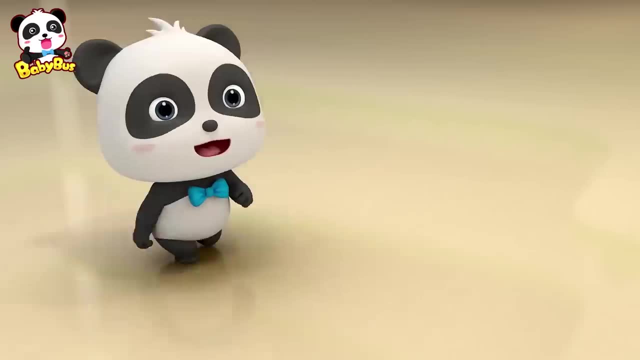 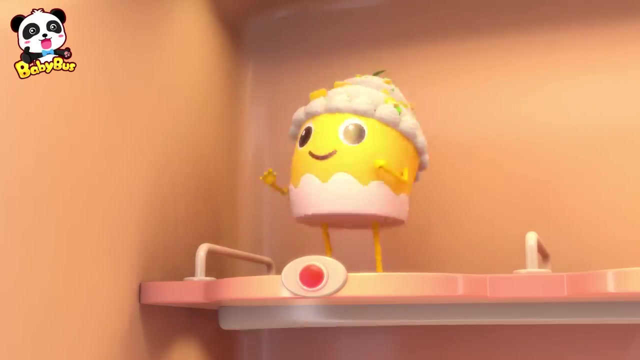 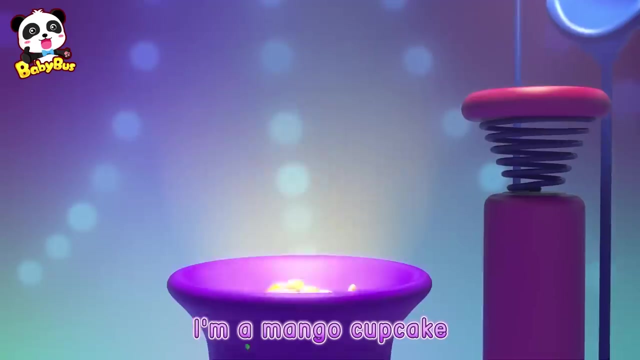 Stand up straight, Wake up. Yeah, Wow, they look so yummy. It smells good. it smells good. The little yummy cupcakes Going down the slide for you, I'm a mango cupcake. Oh, Oh, Oh, Oh, Oh Oh. 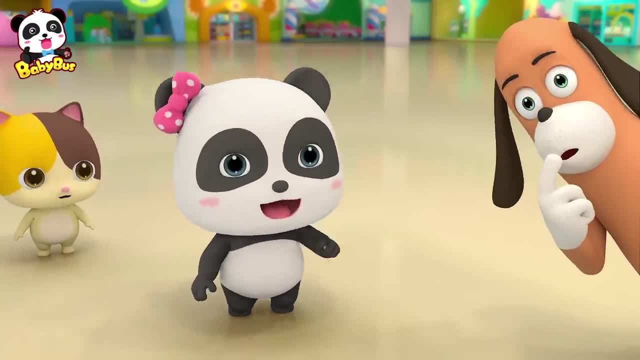 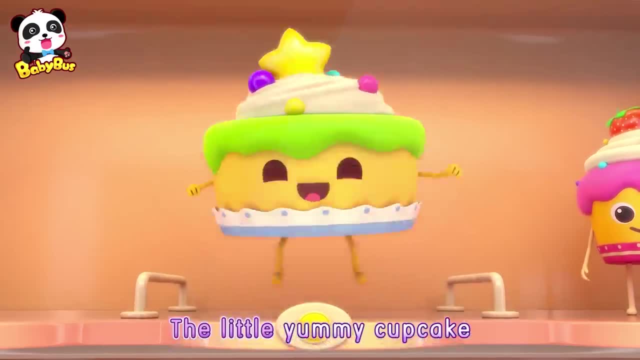 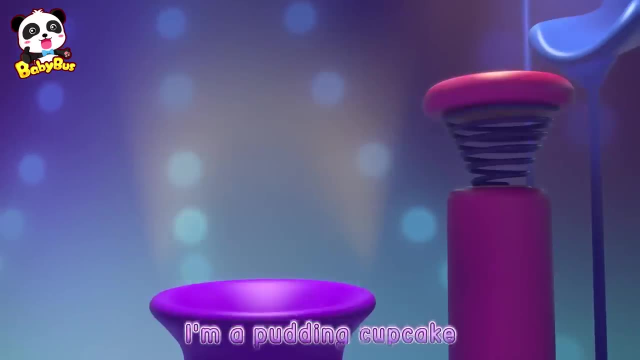 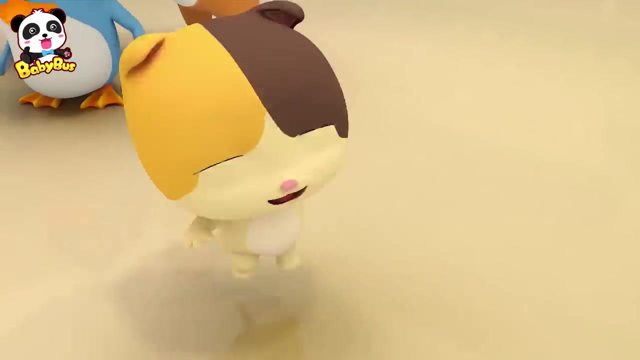 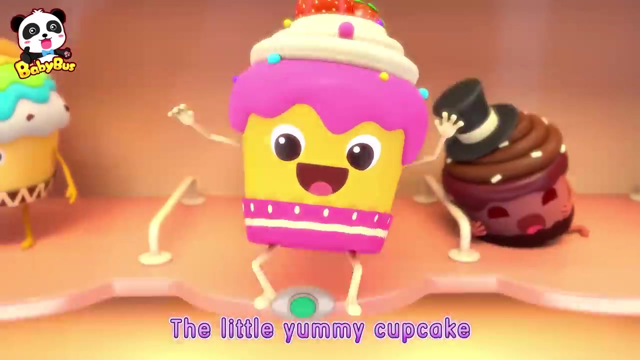 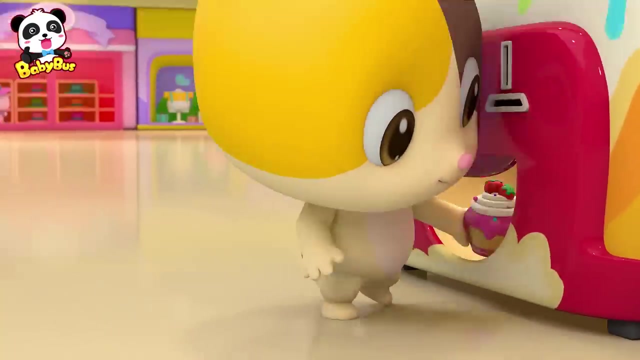 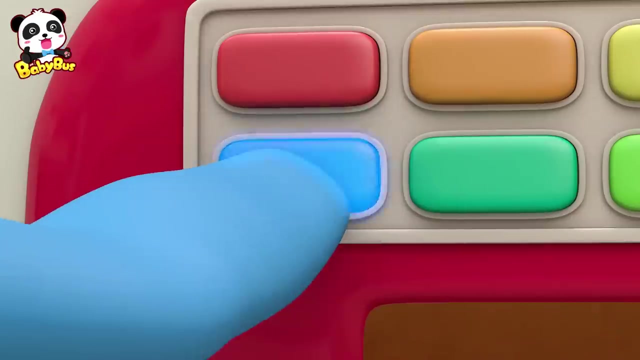 It smells good. it smells good, The little yummy cupcake Going down the slide for you. I'm a pudding cupcake. It smells good. it smells good, The little yummy cupcake Going down the slide. for you, I'm a strawberry cupcake. It smells good. it smells good, The little yummy cupcake.